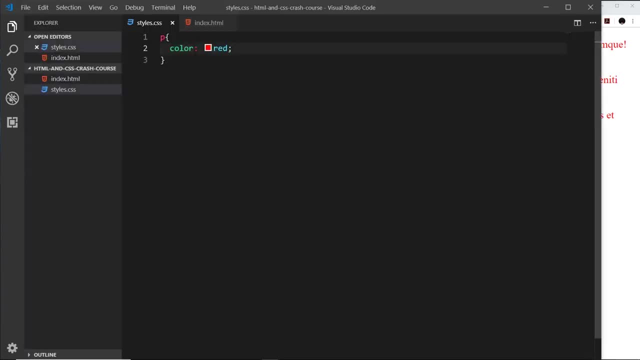 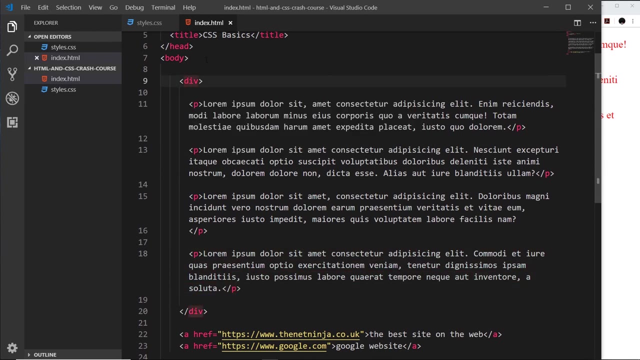 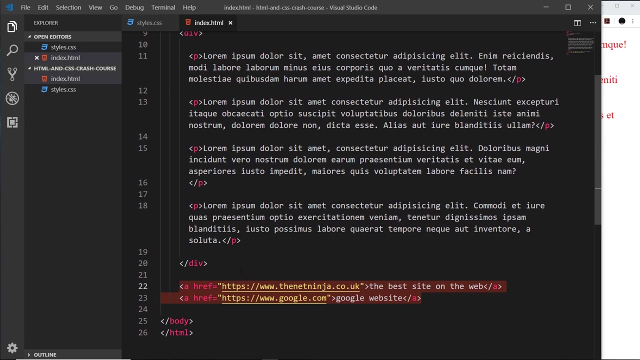 that every paragraph tag now is red. Okay, so what if we wanted to target just one paragraph tag? and, by the way, I already pre-made this HTML template. I hope you don't mind. It's just a div with several p's and also a couple of anchor tags at the bottom. Dead simple, But anyway. 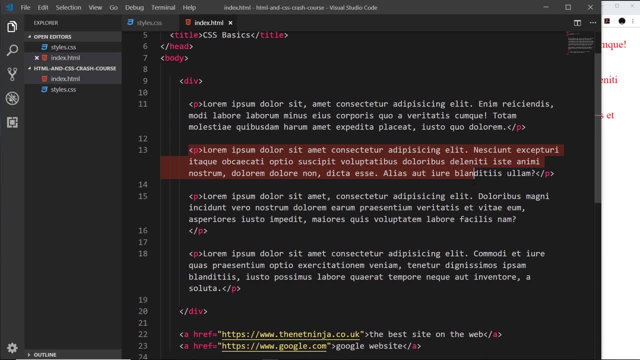 what if we wanted to style, for example, just this p tag? How would we do that? Well, we can use what's known as a class attribute in HTML, and that provides us with a hook for CSS to hook into that and use it as a selector so that we can style just that element with that class. So to do that, 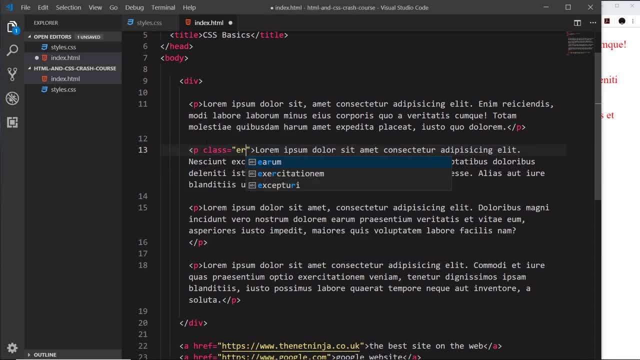 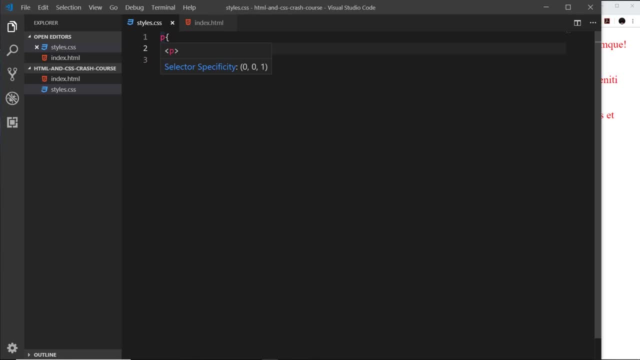 I could say: class is equal to error, like so. And if I save this, then go over to the styles. If I want to target a class, then what I would do is, instead of just saying p, which targets all the paragraph, 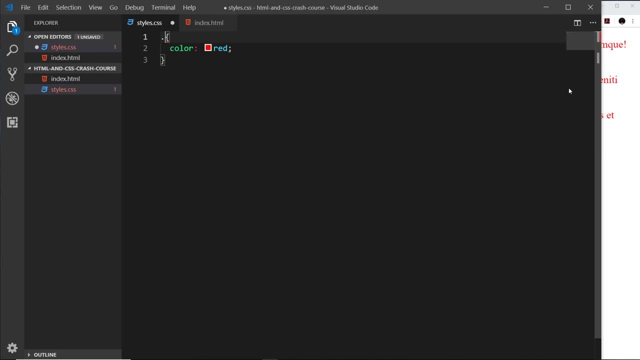 styles, I'd say dot and then the class name, which is error. So if we're targeting a class in a selector, then it starts with a dot. We always start with a dot when we're looking for a class or a period- however you like to call that thing- And then the class name, which is error. 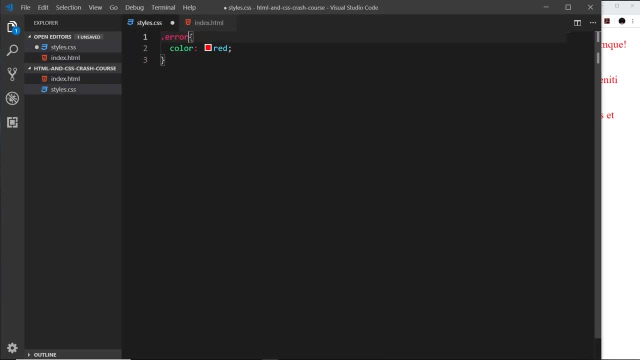 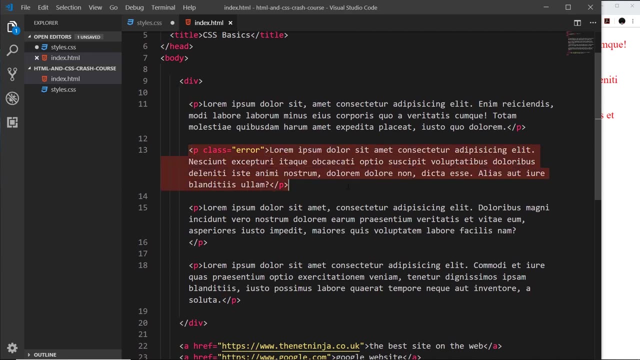 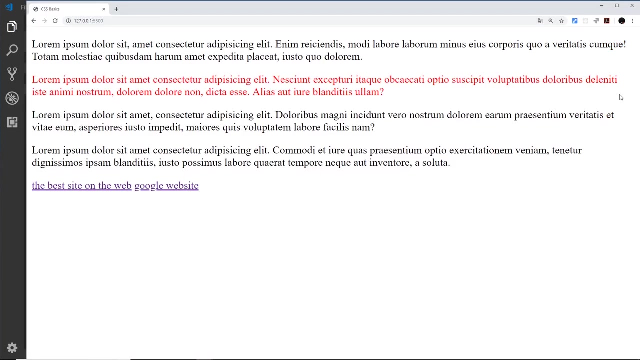 in this case, right here. So what this is going to do is say, OK, I'm going to select anything with this class and color that red. Now, since this is the only thing with that class, it's just going to style this one paragraph red. So save that and save your CSS, and come over here And we can see. 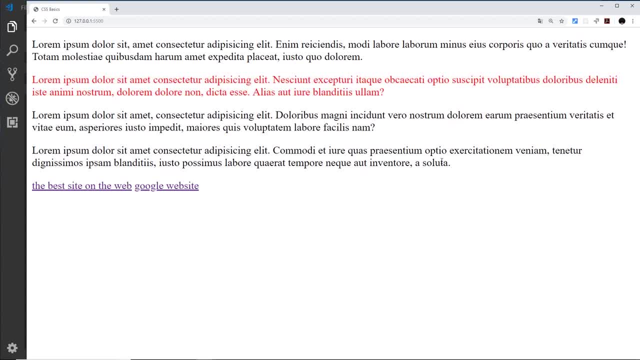 now, just this one paragraph is now red, Awesome. So that's why we use classes: to kind of provide these hooks that we can reach into from our selectors. Grab certain things to style. Now, if we wanted to, we could add this same class over here to: 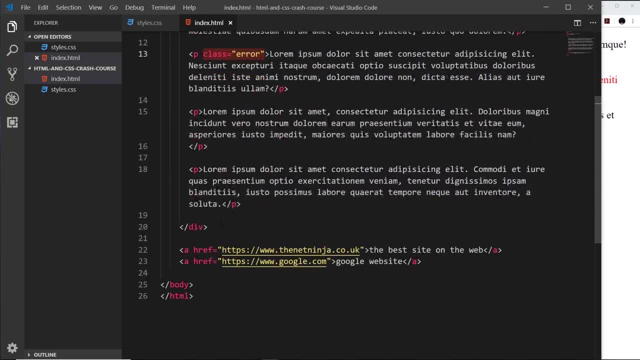 different things. For example, if I copy that and then below this div I just create another div and I'm going to give this a class attribute as well, I'll paste this in and that is also going to have a class of error. Let me just write something terribly original in here. I am an 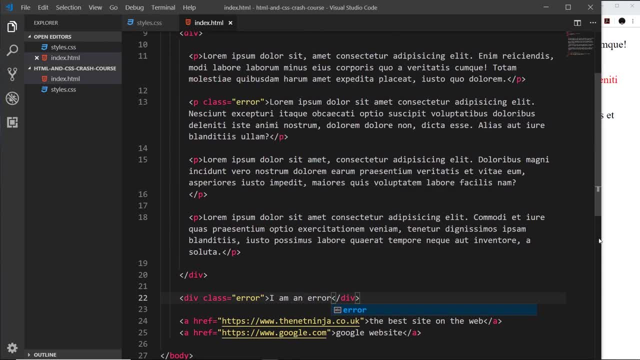 error and save it. Now what do you think will happen? Well, over here we're looking for the error class. Now we have two of those on the page. We have this one and this one. So this selector is going to hook into both of those or select both. 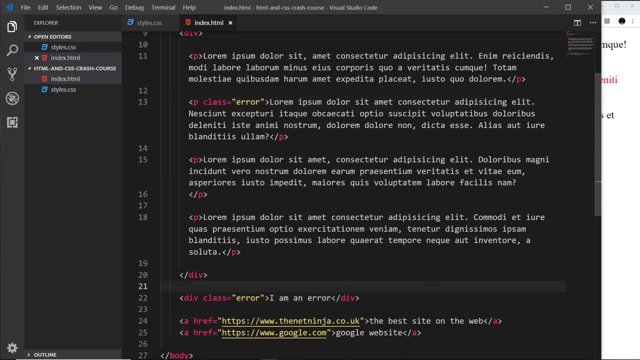 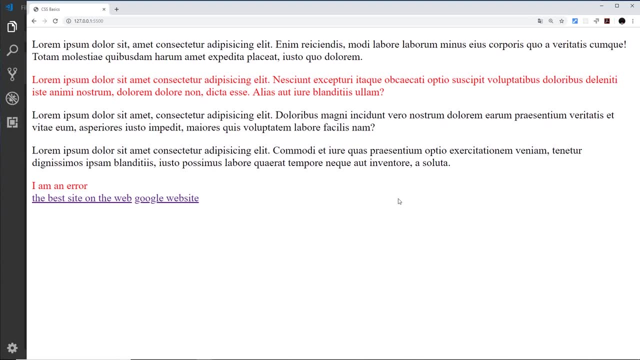 of those elements and style both of them. So if I save this and preview over here, we now see I am an error is also red, as the paragraph is also red. So that's how we use classes. We can add the same class to many different elements on a page And this would be good because you might have a class. 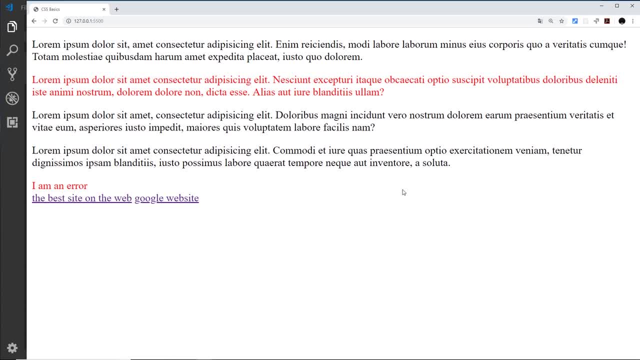 something like CTA button, which stands for call to action button, And with that class you could add certain styles like the background color of the button, the font size, the text color, all that kind of stuff, And then you could apply that class to every button which was a call to. 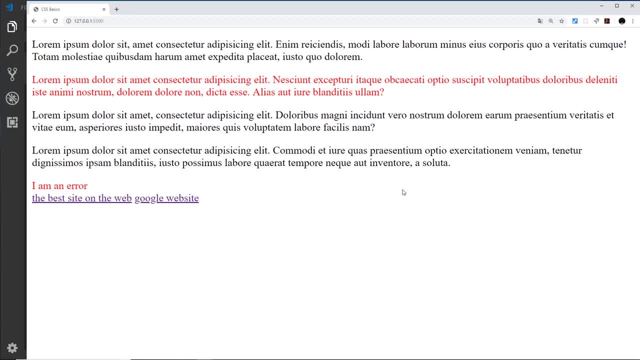 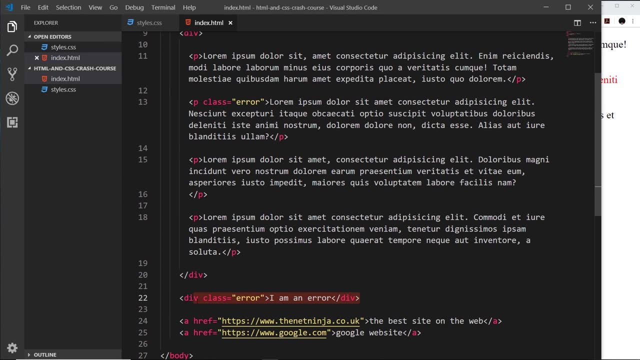 action on your page And they're all going to be styled the same then. So that is a fantastic time saver. It's really good to be able to do something like that. So we've seen classes now. But what if we now want to only get the peas with a class of error So say we're not concerned about this down? 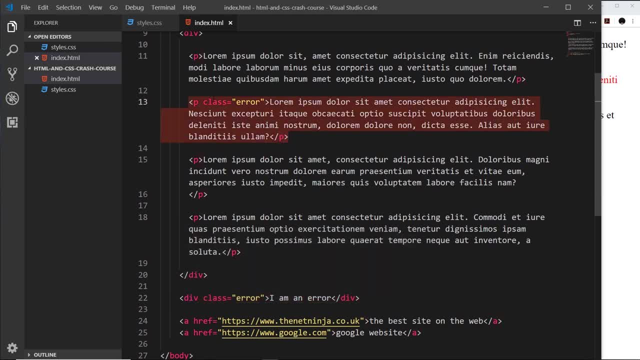 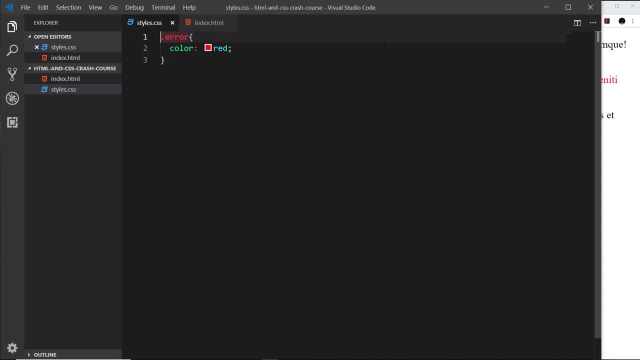 here We want to style the error, but we only want to style Any tags which have that class. Well, what we do in this case is, first of all, we say the element selector, which is P, then dot error And there's no space in between the US, And we're saying OK. 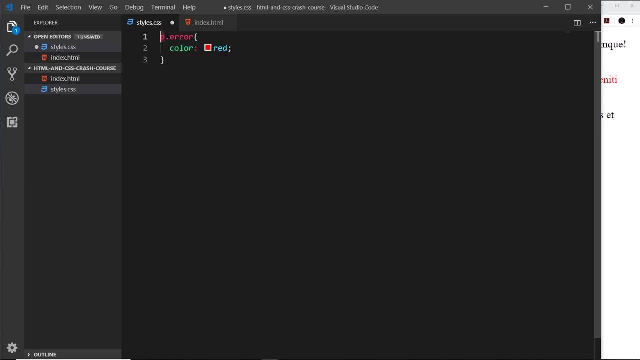 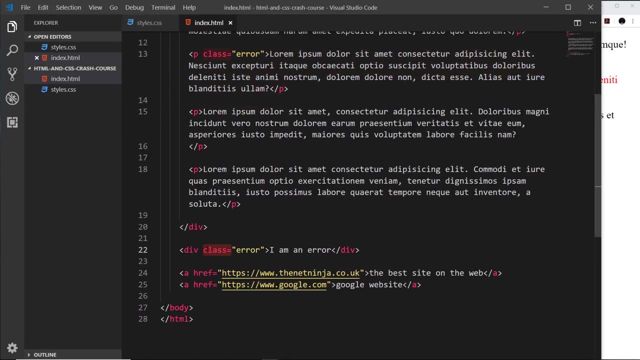 well, look for any tags which have a class of error like this. So now, if I save this, only one tag has the class of error and this is not a p tag, so it doesn't style up. So let me preview, And now we can see this thing over here, just that. 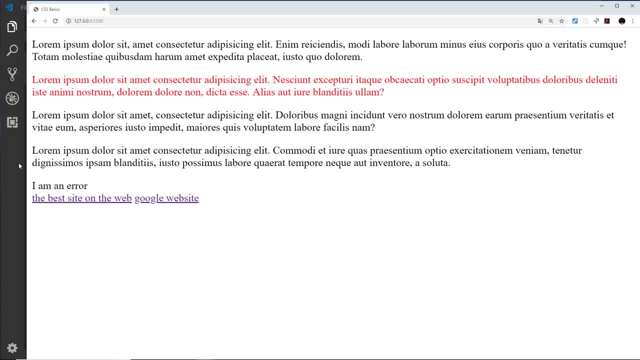 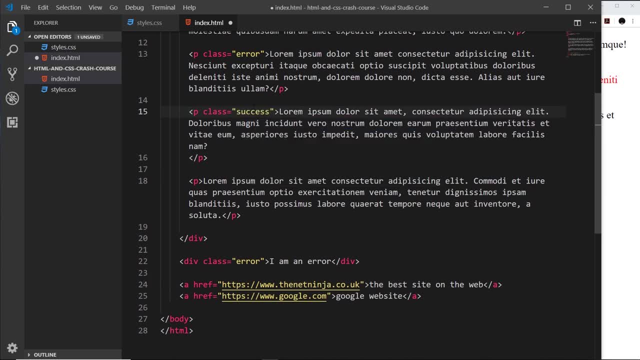 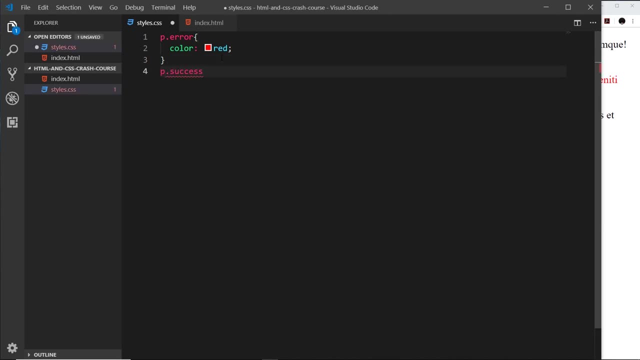 This is no longer a class of error red. all right then. so let's do another little example. I'm gonna give this one now a class of success, so a different class now, and what I'm gonna do is come over here and say P dot success, so any P tags for the class of success. I'm gonna 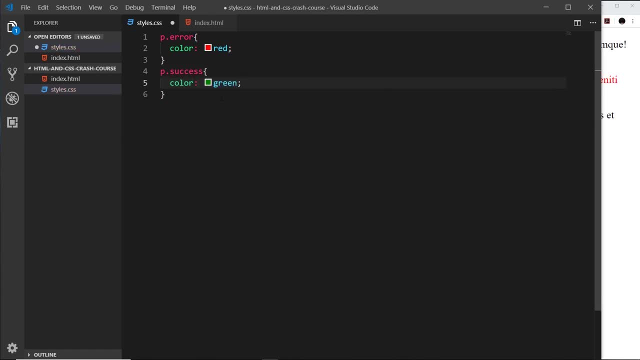 color those green, but what I'm actually gonna do is just hover over this and get a better shade of green, so I'll get the hex code and then come up here that looks like a better green. I'm gonna save this and we should see this one. 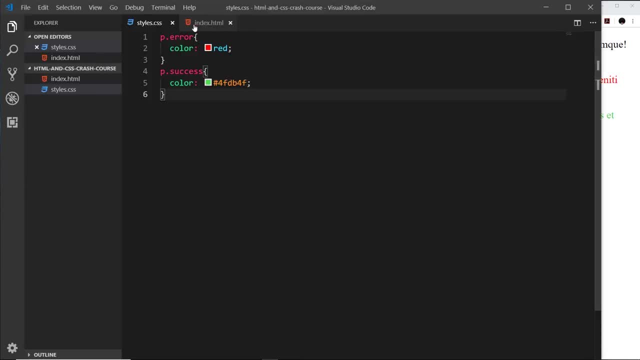 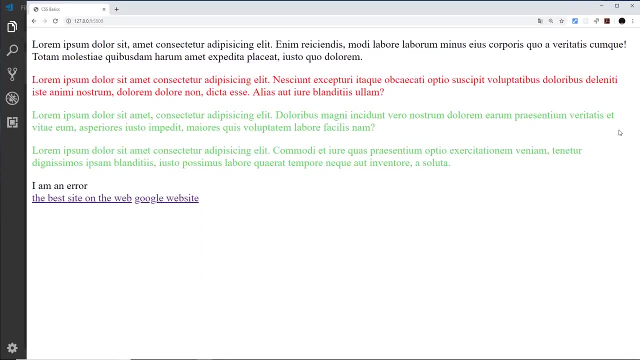 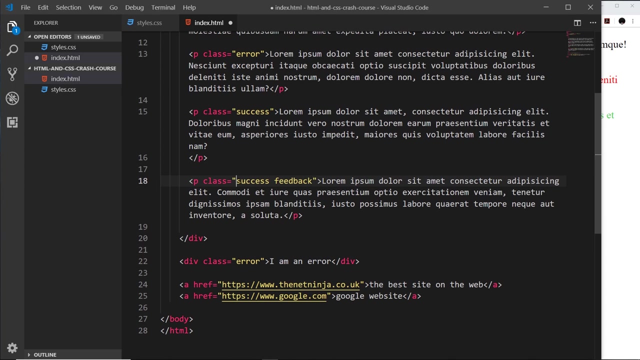 paragraph is now green. awesome. now what if, also, we want to give this a class of success? well, that should be green as well. right, cool. and now what if I also give this a class of feedback? so this now has two classes: the first class, then a space, then the second class. we don't do another set of quotes, they all go in. 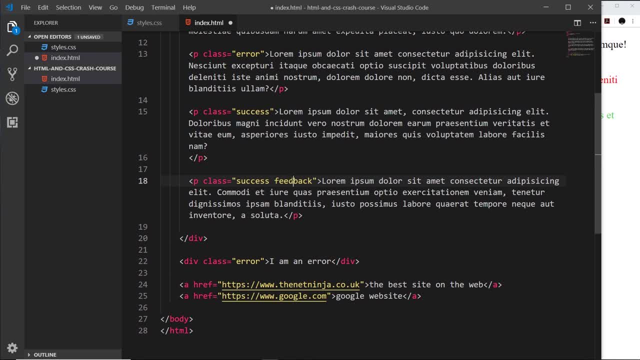 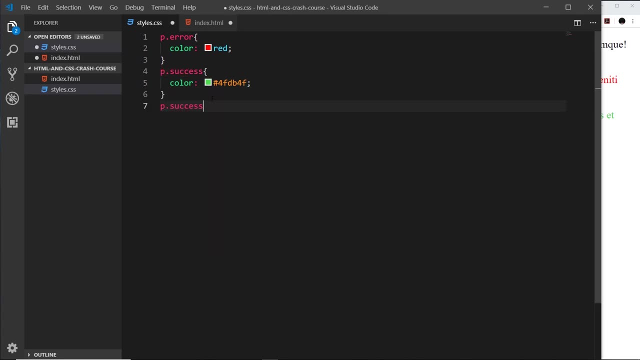 the same set of quotes. we're just giving this now multiple classes. so what if I now want to style all of the P tags which have both of these classes? well, I can do that as well. we just chain them together, much like we have done here. I could say P, dot, success, dot, feedback. so now we're saying: look, 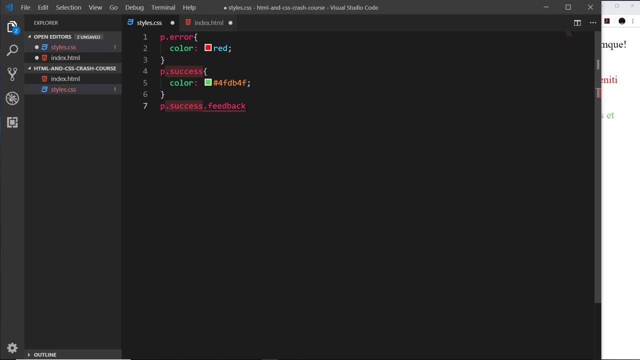 for any P tag with a class of success, with a class of feedback as well, it has to have both of these classes. so we're joining all of these things together. that's absolutely fine, and this time what we'll do is give this a border, and the border is going to be one pixel dashed, and it's also going to be this: 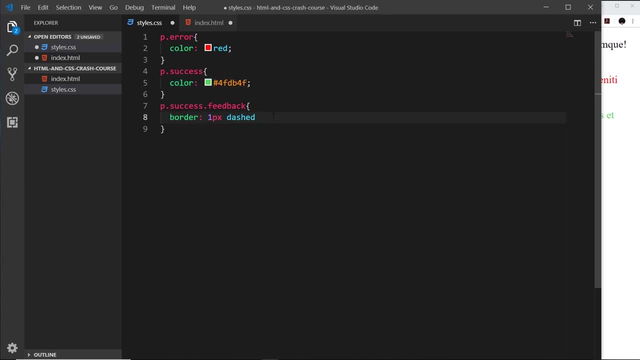 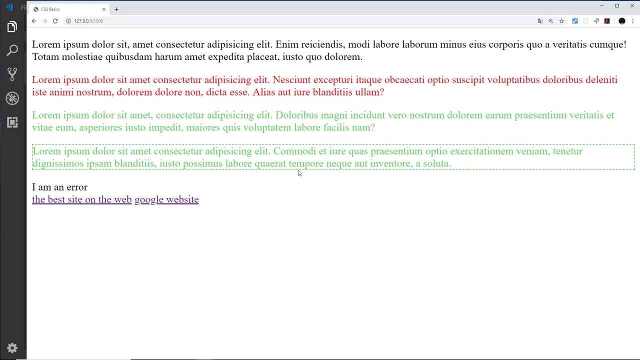 green color right here. so let me paste that dude and save it. cross your fingers, and over here we can see that that has not worked because we've not saved the index. so let's save that and now we can see this border right here. okay, so hopefully that gives you kind of all right understanding of classes and how. 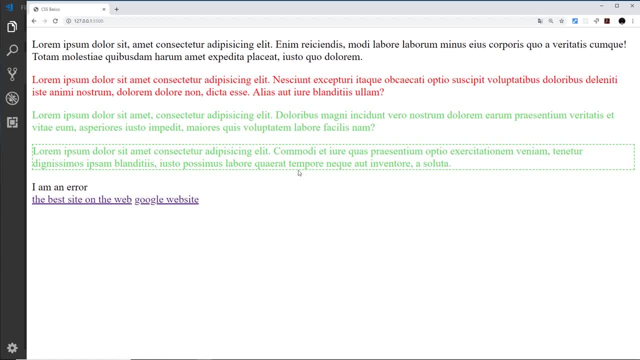 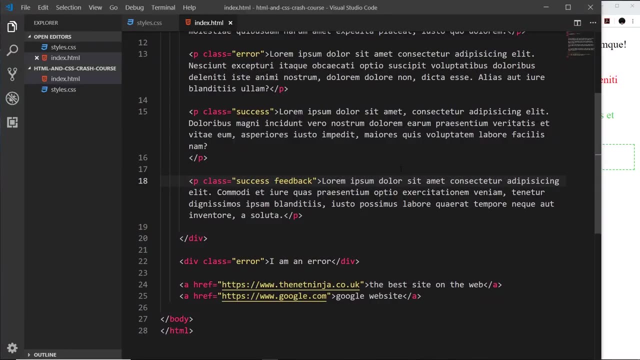 we can use these classes to reach in and get the results that we want to get and and select elements from our HTML to style those. now we've also seen in a past tutorial IDs. we looked at those when we looked at forms. now IDs, I said at the time, can also be used in CSS and they can be used in CSS as hooks. just 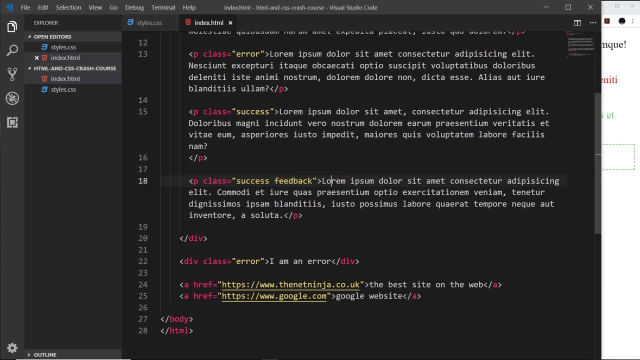 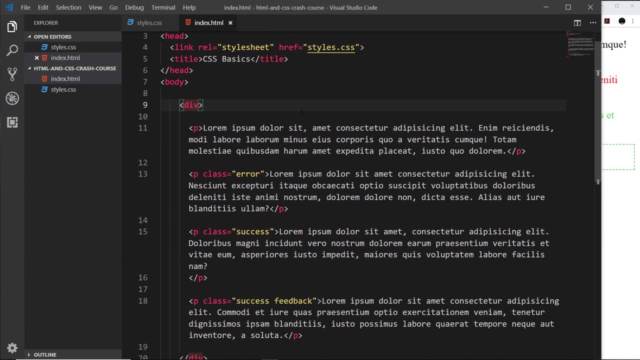 like classes can be, but the more commonly used in JavaScript and that's what I tend to use them for. but you can still use IDs as CSS hooks as well, so what I'm going to do is use that here just to show you and then going forward, I'm rarely going to be using IDS for CSS, so I'm going to say ID. 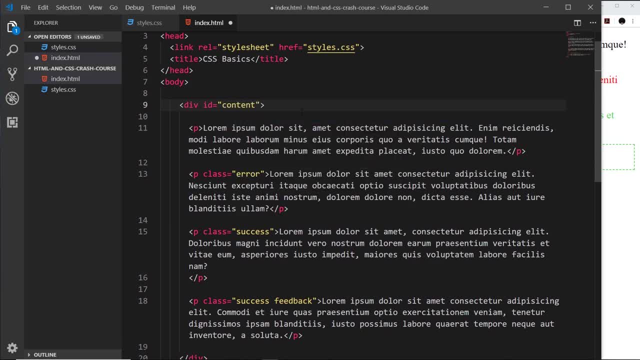 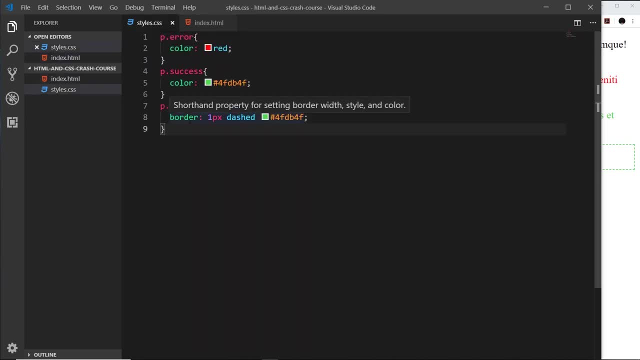 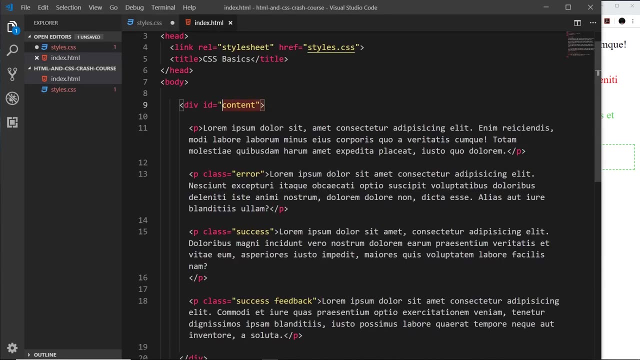 is equal to content. we'll call this. I'm gonna save that and then, if I want it to target an ID from a style sheet, all I need to do is say hash, which stands for the ID. then the ID name which I said was content. that's what we called it, right. 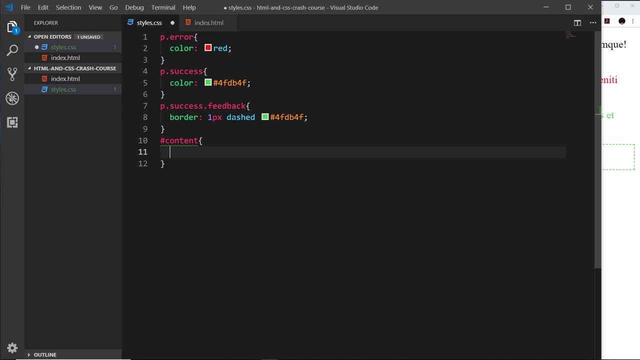 here, and then we just open up our curly braces and do our different declarations. so I'm gonna say background color is going to be eb, eb, eb- i know that hex code, it's just light gray. and then i'm going to say padding is going to be 20 pixels all the way around. so if i save this now, then we're going. 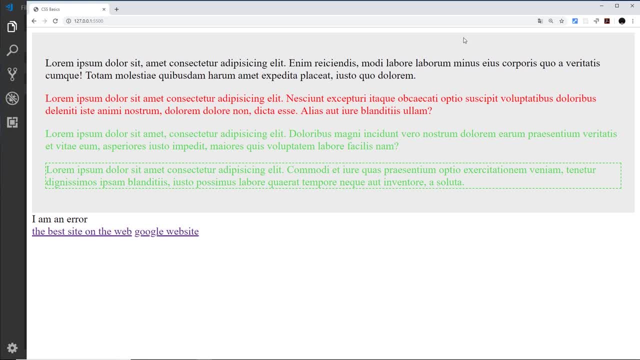 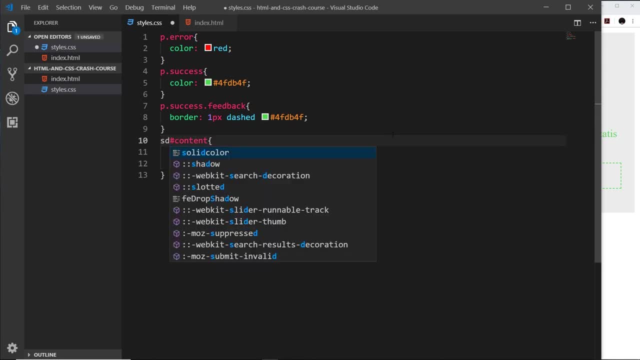 to see. it's targeted, that div with the id of content, and it's applied. those styles now same again. if i wanted to make this more specific and say, okay, we'll just get the div with an id of content, then i can just put the div in front of it, much like we put the p in front of the class. 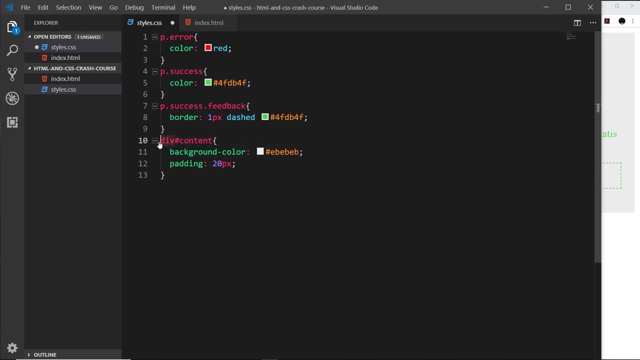 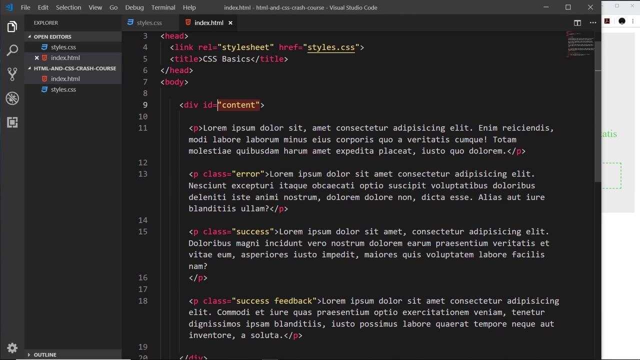 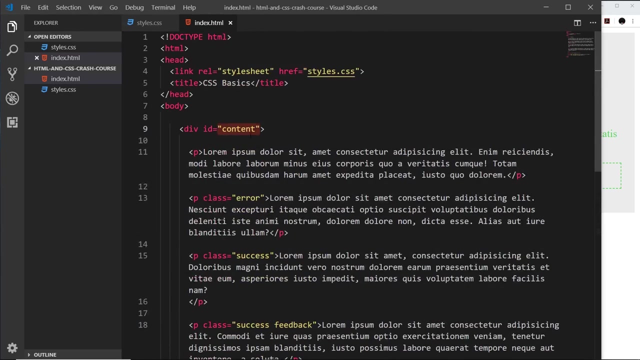 okay, so the one constraint that ids have is that you can only use one id of this name on each page and not just this name. what i mean to say is all ids must be unique, so i couldn't use content anywhere again as an id on any other element and if i called this something else, like something, 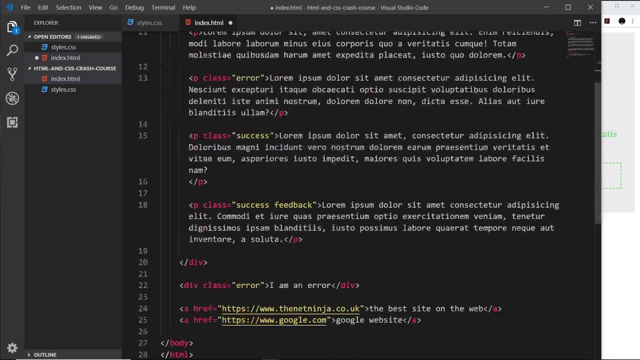 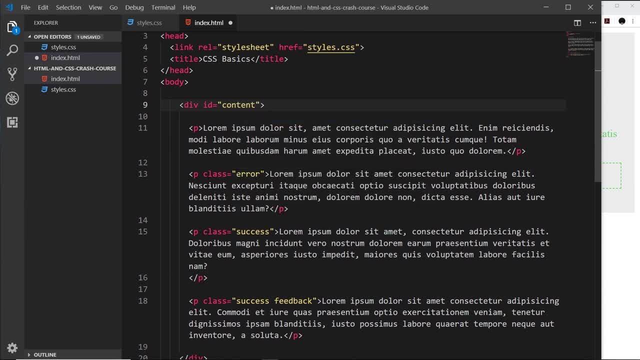 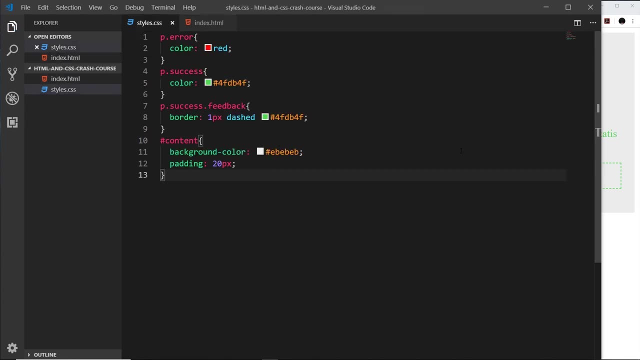 use ids for css hooks. i tend to stick with classes like this because they do the job for me and i only really use ids for javascript. but if you want to use ids, there's nothing stopping you. you can certainly do that. it's just a style that i adopt. so then, another way to be more specific with what. 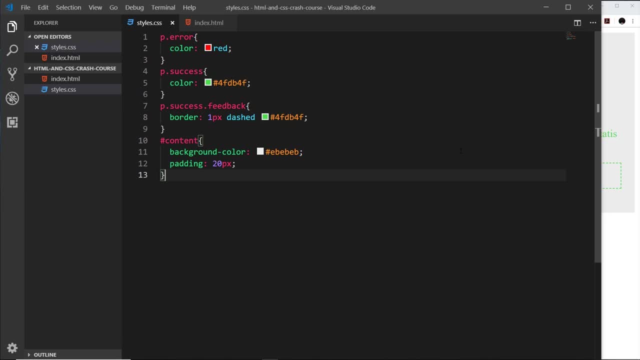 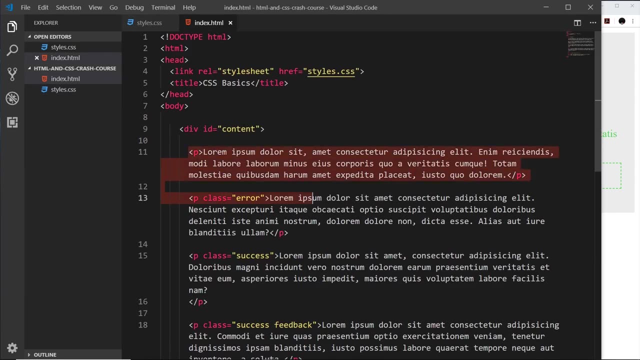 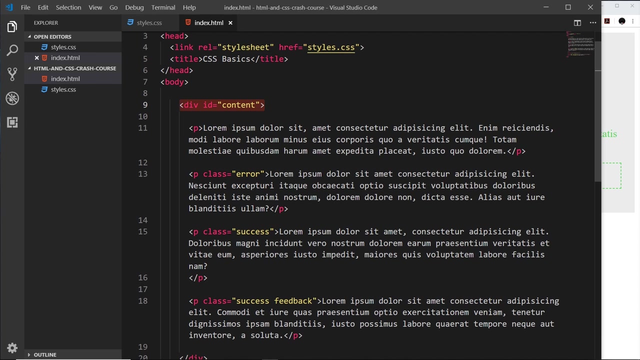 elements we want to style is by using what's known as descendant selectors, and this means that we can basically target children inside a parent element. so these are children right here inside a parent. they're nested inside of them. so if i wanted to target p tags, but only p tags, 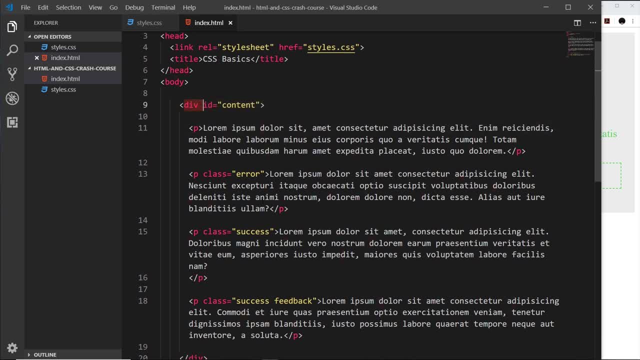 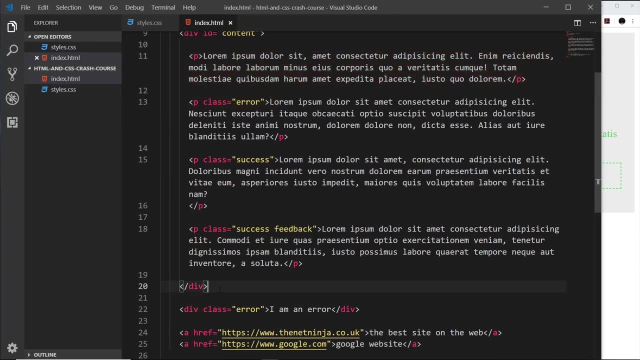 nested inside a div like this, then i could do that with a descendant selector. now i know that these p tags are the only ones on the page, so there's no point in doing this. but, for example, if i did another p tag down here and, by the way, to get some dummy content quite quickly, you can just type out: 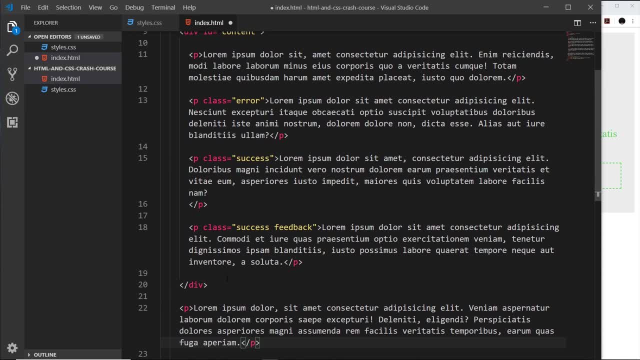 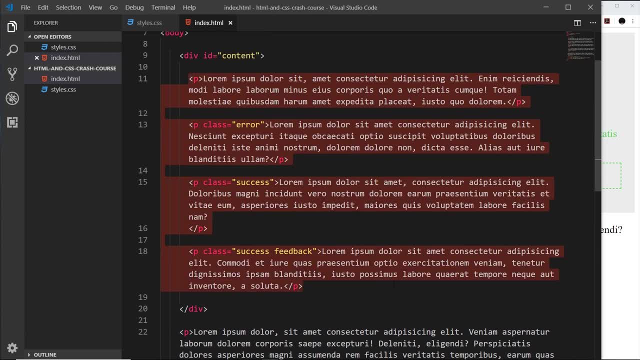 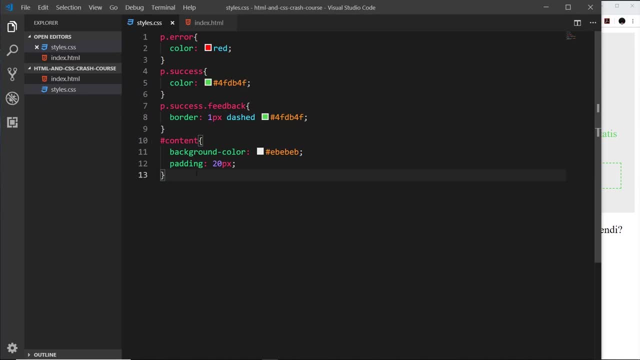 want to target p tags, but only ones inside a div. i can use a descendant selector to grab those and not this one down here. so the way this works is, first of all, we say the parents- and in fact i'm going to comment all of this control forward, slash out, so it doesn't have an effect. so we say the. 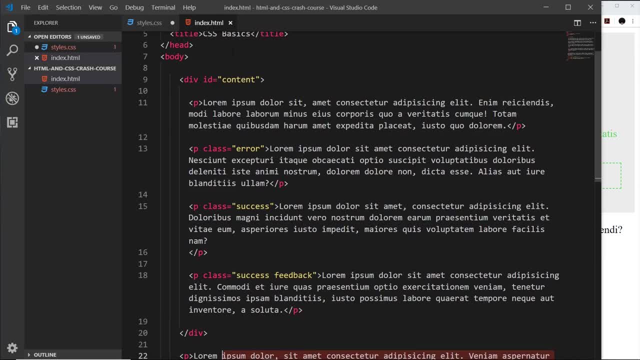 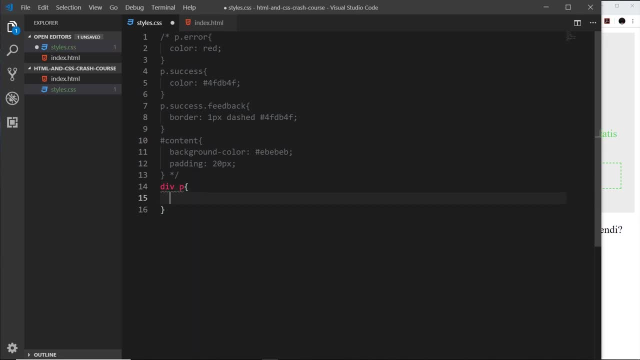 parent first of all in our selector, which is the div, that is the parent right here. yeah, then we've the child, we have a space first of all, then the child, and then open up our curly braces, then we do our declarations. so i might say in here something like color is going to be purple. 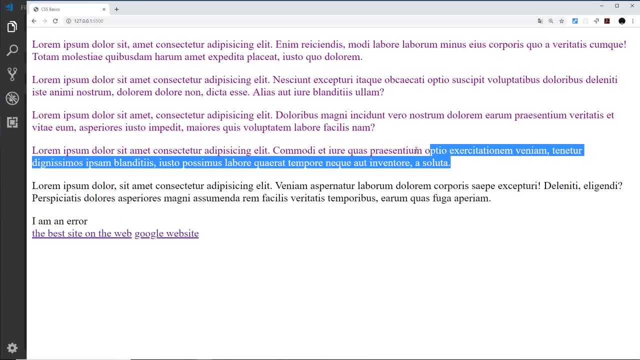 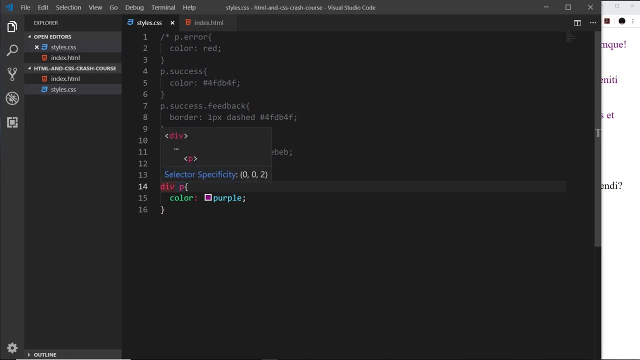 okay, save that and notice now. all of these are purple, but this one is not, because it's not inside a div, so that is a descendant selector. we say div, the parent goes on the left and the child on the right, and we could do this several layers deep if there was something else in the p tag, like 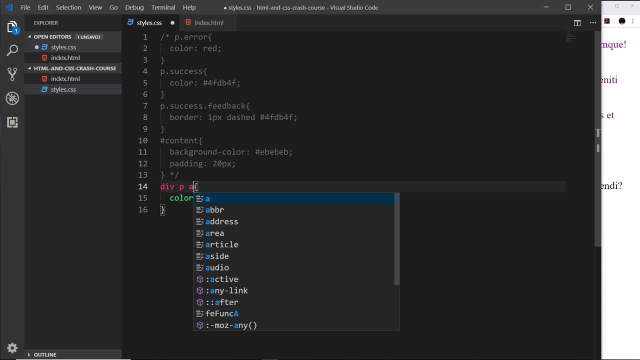 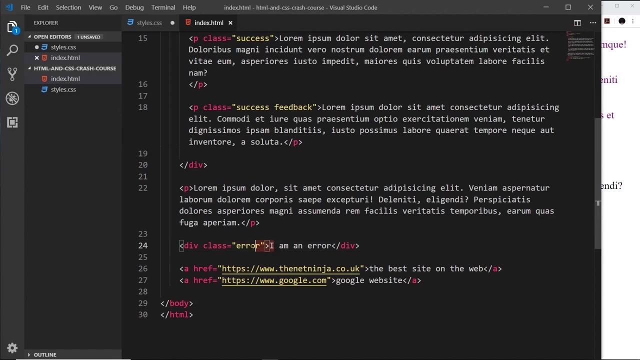 an a. we could target that as well, and then this would only target anchor tags inside a p tag, inside a div tag. okay, now we could get more specific. we could say: we only want to target errors inside a div tag. remember, we have this thing right here, we have this thing down here as. 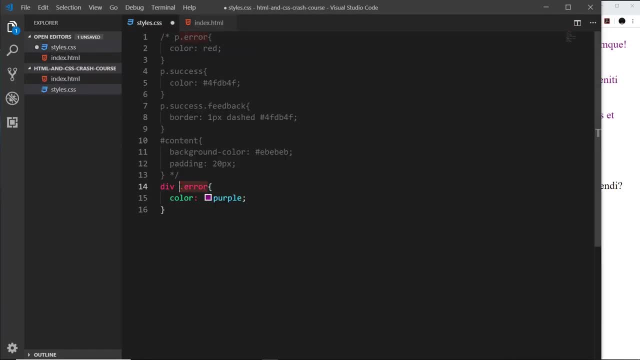 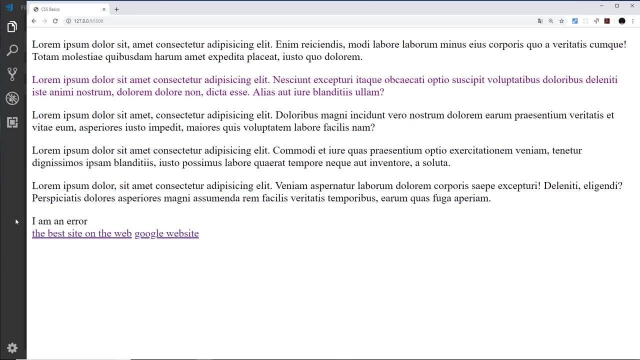 well, now we're saying we only want to target the error class if it's inside a div. so if i save this and refresh, notice this: this is the only purple one right here. you can't really tell the difference that well, so i'm going to turn this to red instead save it and preview. okay, now, notice the space right here. 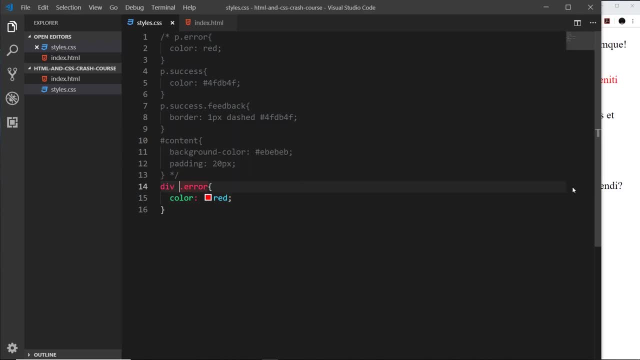 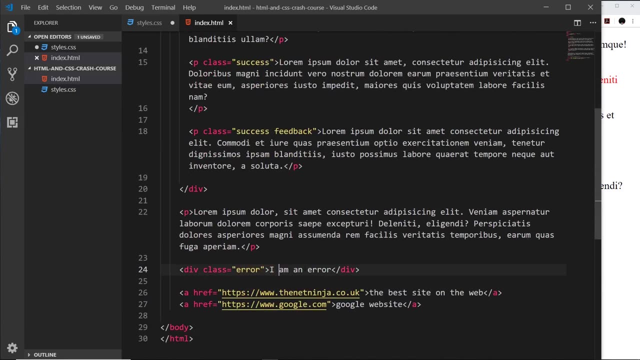 between the div and the class of error. if we were to remove that space, we're now saying, okay, well, get the div with a class of error attached to it, and that would in fact get this thing down here: a div with a class of error, but by adding a space we're saying this is a descendant selector. look. 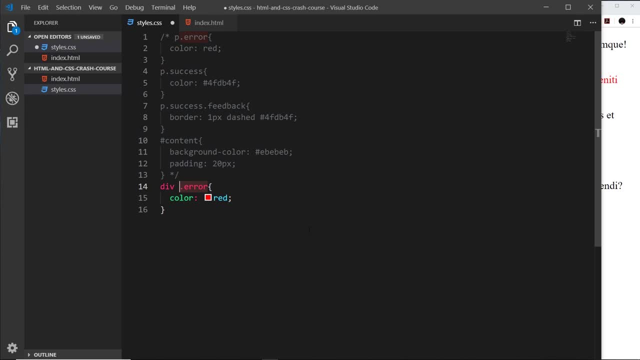 for the parent div, then gets any class of error inside that div, any element with that class of error, and style that okay. i hope that makes sense. so the next way i'm going to show you how to select elements is by using what's known as attribute selectors. now we've already seen what attributes 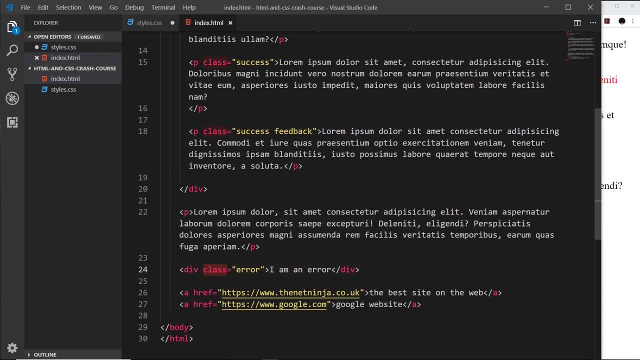 are in html. things like these are an attribute: the class that's an attribute, this is an attribute, href and any other kind of attribute that goes in here. we can use those as selectors. so say, for example, i wanted to select an anchor tag or every anchor tag on the page which had this attribute. 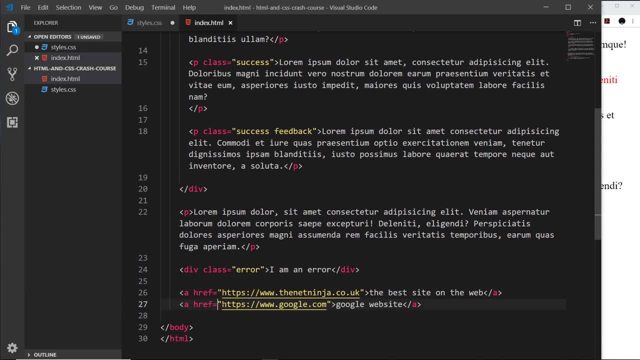 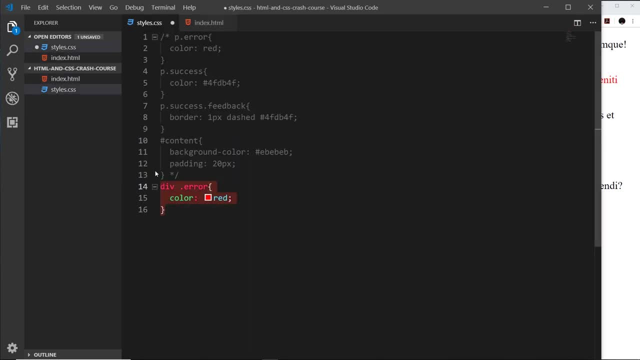 href right, doesn't matter what the value of the href was, it just had to have this href attribute. then i could do that. so i could say: okay, let me comment this out. first of all, i could say: find every anchor tag. then i use square brackets. this is to use an attribute selector. then we put: 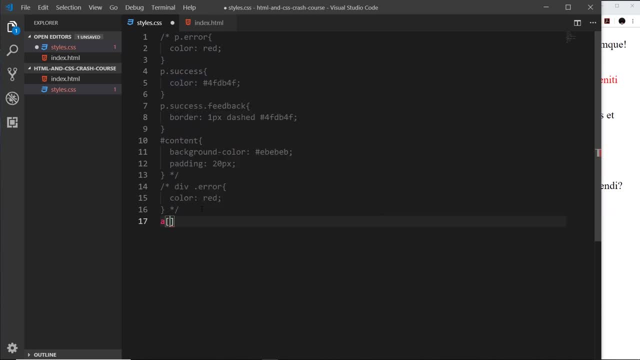 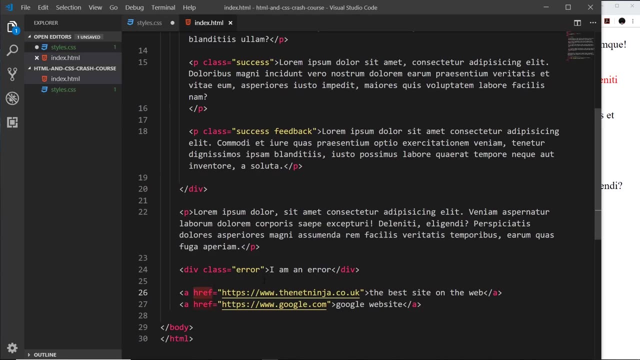 the attribute name inside these square brackets, which is just href. so that is going to look for every anchor tag with an href attribute. now, most will do so, probably going to target 99, if not more, of the anchor tags on your page, but i just wanted to demonstrate this. 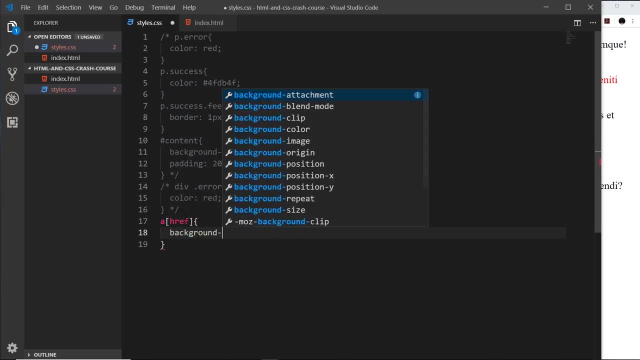 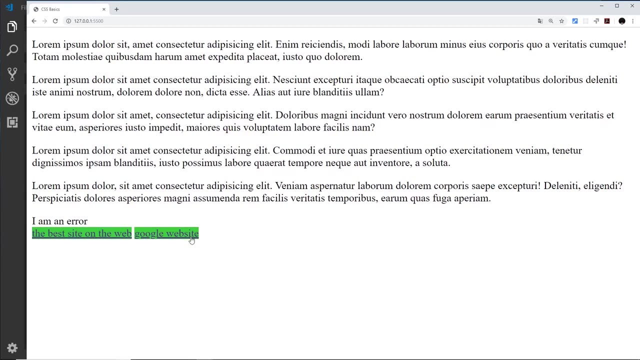 so i'm going to now say: background color is going to be this hex code that i found before. it's a greeny color, so if i save this, then we should see that every anchor tag now that has an href attribute is colored this color in the background. okay, so what if? 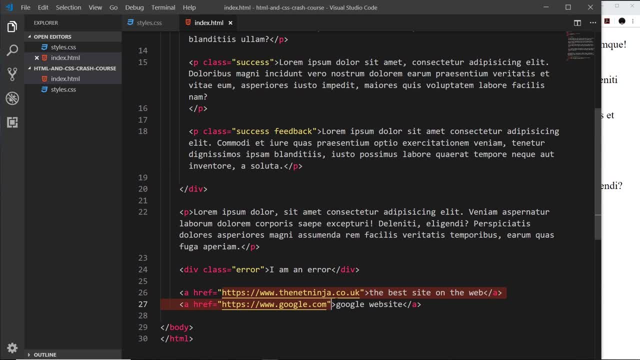 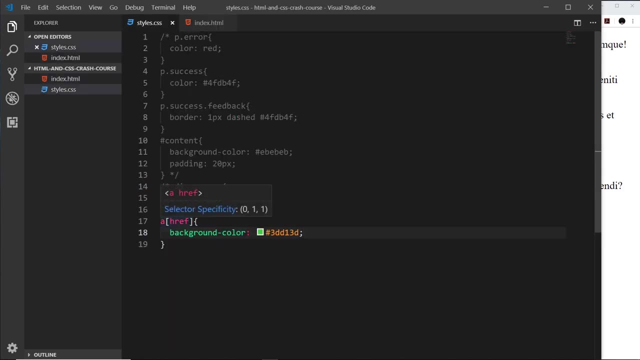 i wanted this particular attribute to equal something. for example, i wanted to style every single anchor tag on the page where the href is equal to this value, right here, the netninjacouk. well, i could do that. i'm going to copy this dude right here, then go to the styles and then all we. 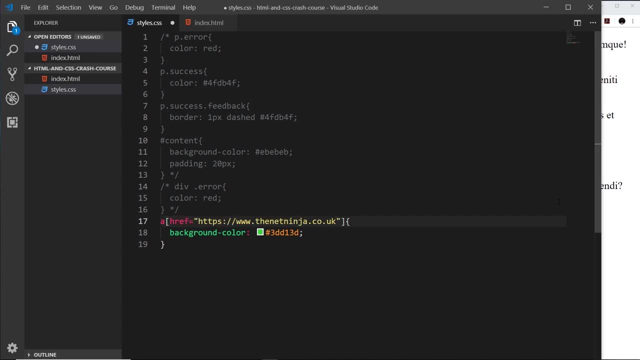 do is say equals, then quotes and then paste it in right there. so now we're saying: select every anchor tag with an href equal to this, right here. so now we're going to give those a background color of this green. not any other tag, just those with an href equal to this. so let me save it and 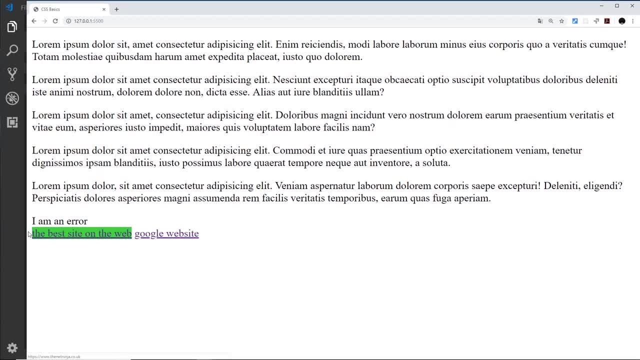 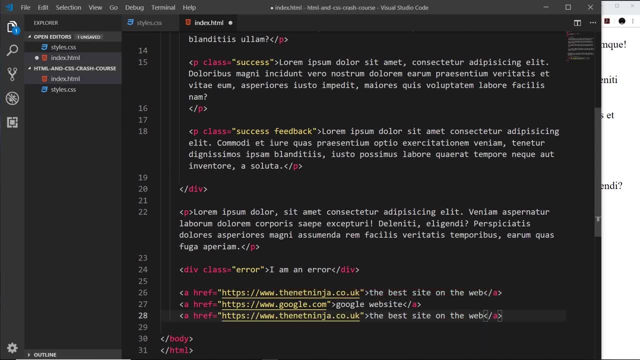 preview, and now we can see only the first anchor tag is styled that way. now, if i was to just copy this and paste it down here as well, then it should style both of those, because they both have this attribute. save it and we can see that right here. awesome. now i'm just going to give these some 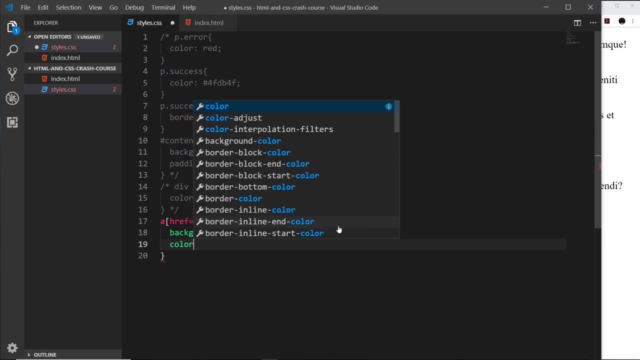 extra styles just to make it look a bit better. so i'll say color is going to be white, that's the text color. and then we'll say text decoration is going to be non, that takes away the underline. and then i'm going to say the front weight is going to be bold. 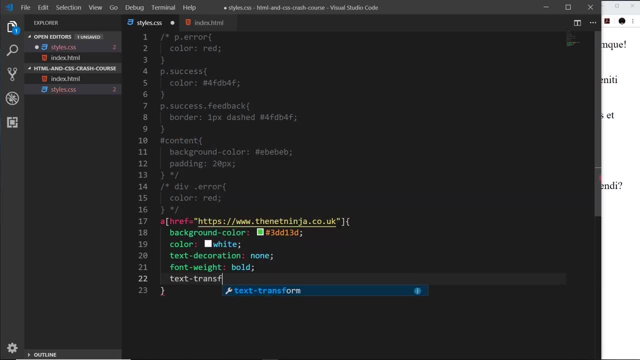 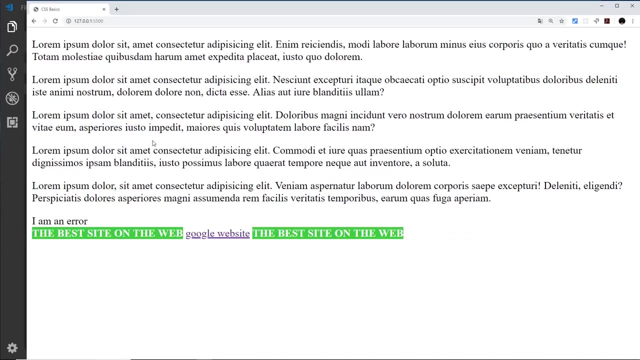 and then, finally, i'm going to say text transform. we've not seen this one yet, but what we can do here is meaning in this example, if we wouldn't have this, if we wereamura today, if this do, is set it to uppercase, like so. so if we save that and preview now we can see. 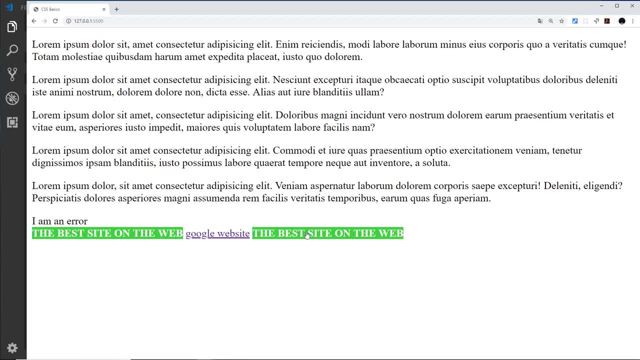 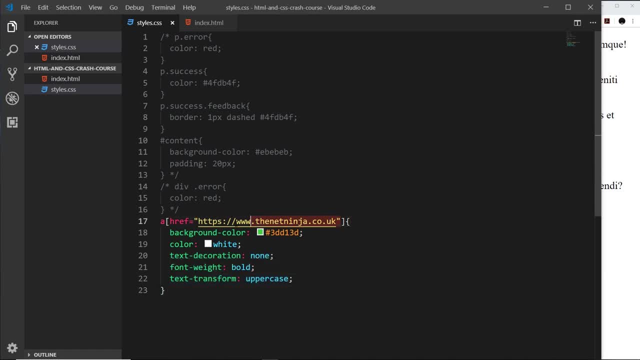 anything with that href attribute, with that value, is going to be styled like this: awesome, okay then. so what if I wanted to shorten this, because this is quite long? well, I could use the asterisk in front of this equal sign. so I could say instead, if I wanted to put an asterisk there, and then equals, and then 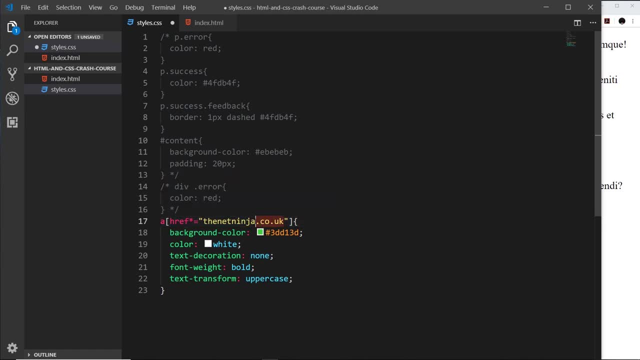 we'll just say the net ninja, like this, and then what this says is: okay, any a with an href that includes the net ninja. so this is somewhere in the value of the href. that's what this asterisk means, that this is included in the value. then 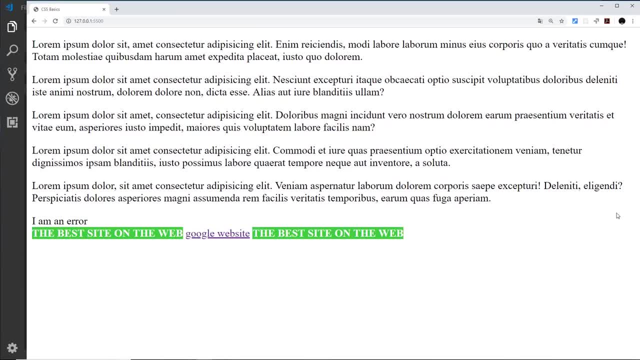 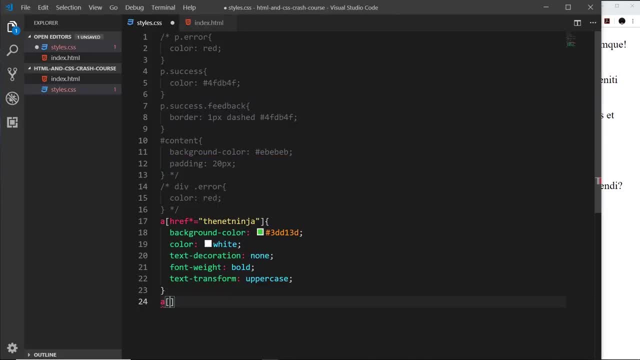 style this way, so hopefully this should still work. let me save that and preview and that works. now I could do something similar. I could say a, and then href is going to be asterisk, a equal, which means it includes something, and I'm going to say Google, and if it? 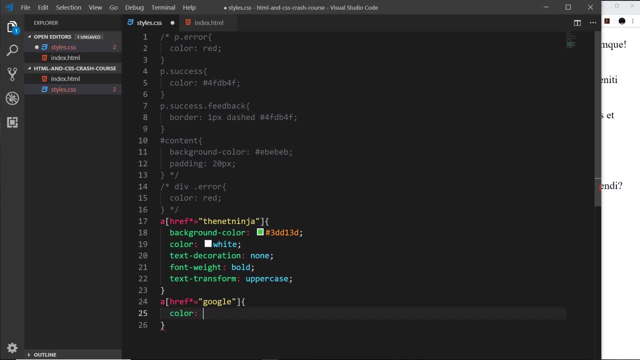 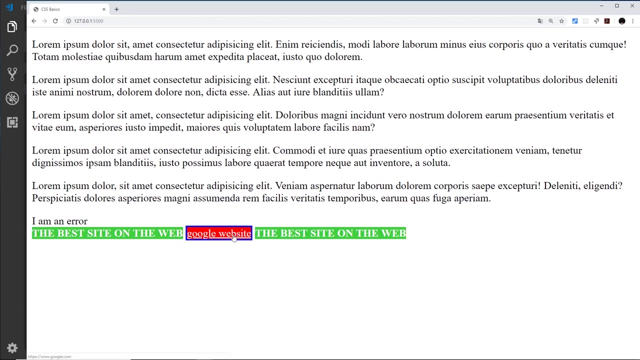 includes Google. I'm going to color this white, give it a background of red and also a border. two pixels solid and blue. okay, so anything that includes Google in the href now, which is an anchor tag. I want you to style this way, so save it, and now we can see this thing right here. 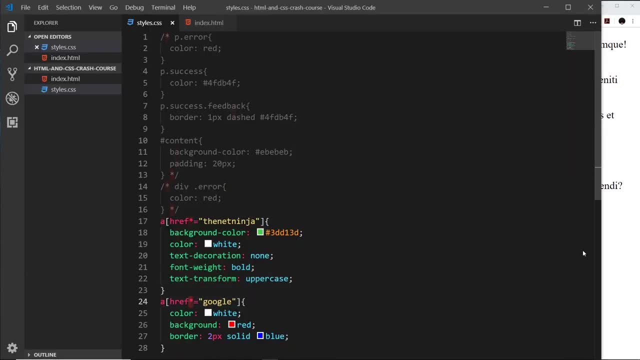 okay, now I can also, instead of using an asterisk, use a dollar and what that dollar means. okay, any href which ends with this: now nothing ends with this. so if I save it, nothing's gonna get styled this way. but this thing right here ends in dot-com, so I could say: ends in dot-com. I want you to style like this. so 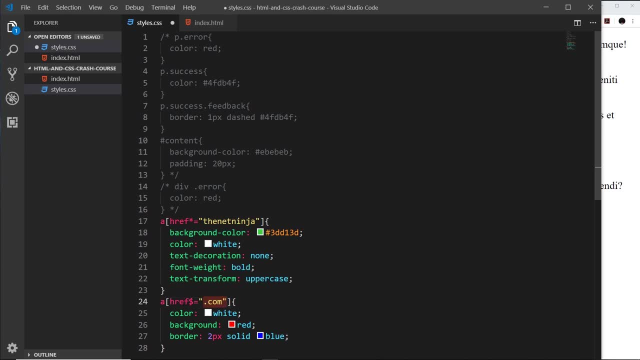 basically any anchor tag which ends in dot-com or the href ends in dot-com. so if I save that on preview then we can see is styles it again. so these attributes selectors are a good way to target elements with specific attributes that also have specific values. remember we can use equals to get an exact match. 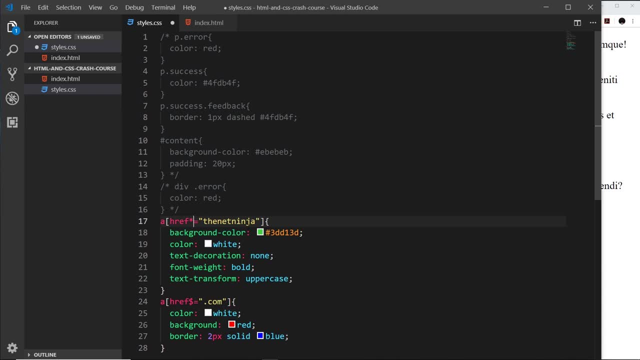 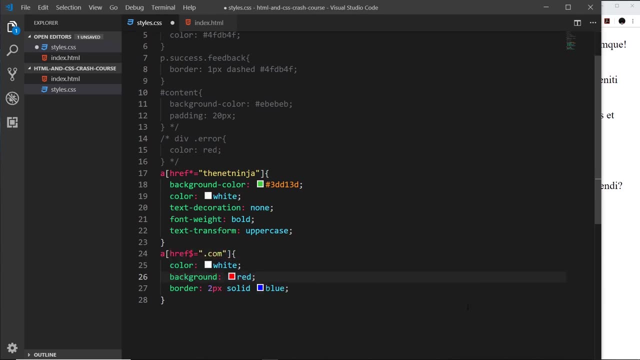 we can use asterix equals to say it includes this somewhere in the value, or we can use this dollar sign equals to say that this comes at the end of the value. so these are really useful for situations where you want to start certain different things with different 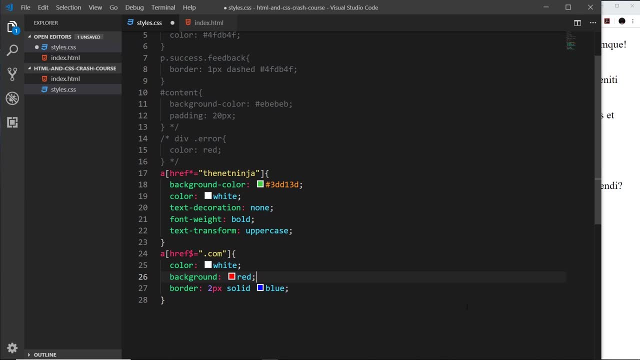 attributes differently. an example of this could be any anchor tag that ends in dot pdf, because that would be a pdf download, and if you have a pdf download you might want to show a little pdf icon next to it. so you could style it that way. you could say: find any anchor tag where the href ends. 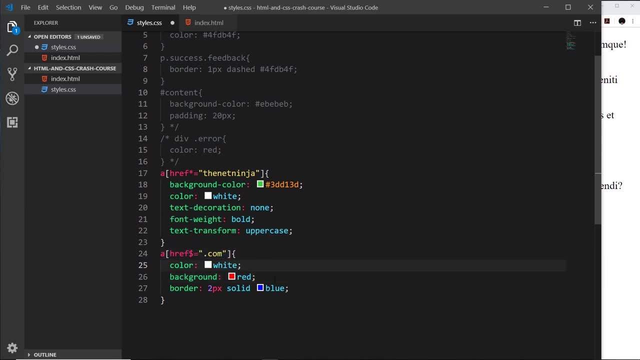 in dot pdf and you could give that a background image to the right of a little icon of a pdf and that would be a nice user experience to see that this is a pdf that they're downloading. so these kind of things can be really useful for all kinds of those situations. 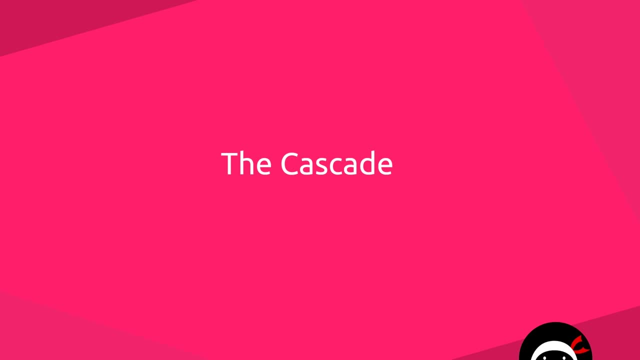 so then, my friends, you've heard me by now talk all about different types of selectors, rules and all that jazz, and i'm sure you're getting quite bored, so i'm going to take a little side step for now and talk about selector specificity and also the cascade which is the c in css. now i don't want. 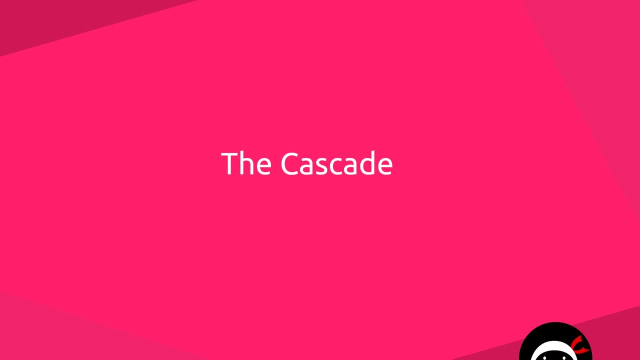 to delve too deeply into this kind of stuff, but it's going to be a little bit easier than it used to. so now we've got a little bit of information here and we're going to talk a little bit about what this? because this is a beginner's crash course and we could end up going down a rabbit hole and 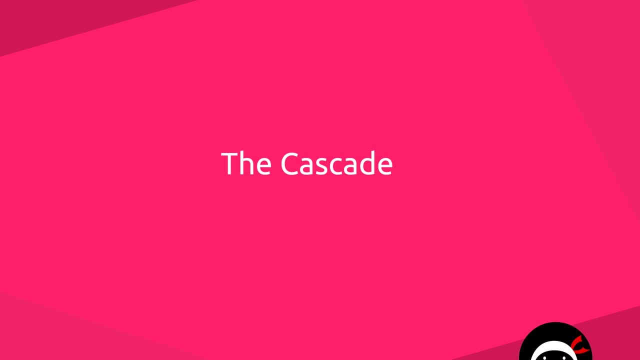 getting deeper and deeper, which I don't want to do, but we will talk about the basics so that you understand this, at surface level at least. So, first of all, this cascade- Cascade as a word in itself means to pour downwards like a waterfall. cascades from top to bottom, right Now the CSS cascade kind. 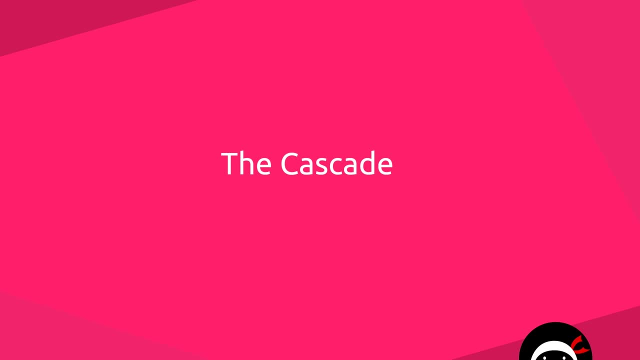 of takes this definition on when it comes to rules cascading from top to bottom. It's all about CSS properties flowing down from parents to children, and it encompasses really two different concepts: inheritance and specificity. So the first thing we need to understand to make this clear. 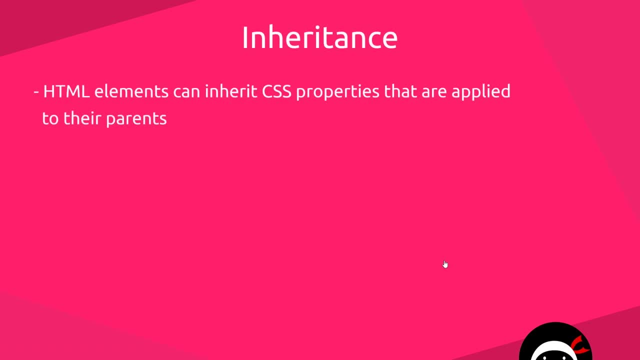 is that HTML elements can inherit CSS rules that are applied to their parent elements. So if we had a code which looks something like this: for example, we have a div as the parent and then a paragraph nested inside it. If we had a CSS rule that looked like this, where it targeted the div, 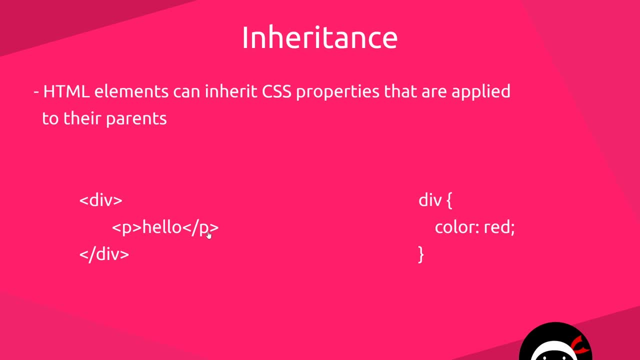 the parent and colored it red, then this p tag would also inherit this property right there. So we'd see red inside this text. The text itself would be red rather, and this applies several layers deep. so if we had another tag inside their span, for example, then also that would inherit the great. 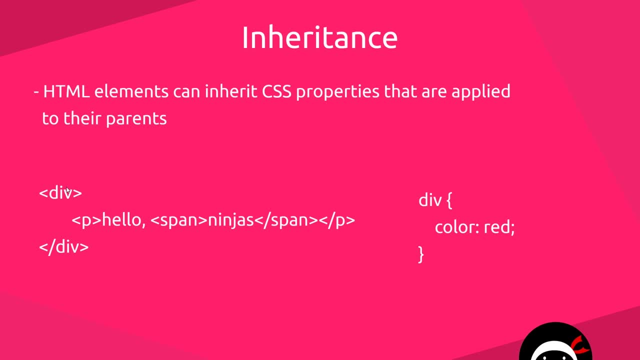 grandparent or whatever it is. you know the parent parent style of this right here, and that would be red as well. So that is inheritance. We're basically inheriting what we style the parents as and it's being passed down to the children. So child elements inherit CSS properties from parent elements and 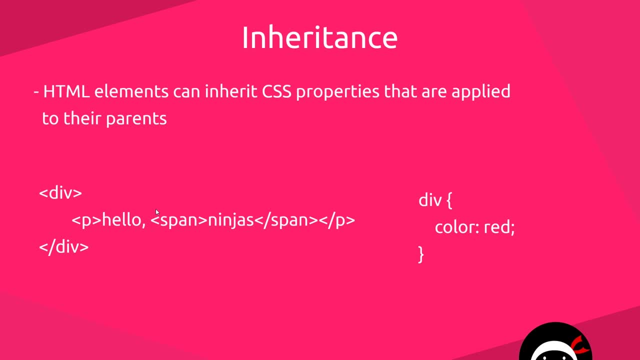 that's called inheritance, but not all properties are inherited. Things like margin padding and background styles and borders- they are not inherited. It's mainly font and text styles or colors that are inherited. So let's have a quick look now at some examples. Okay, so now I want to. 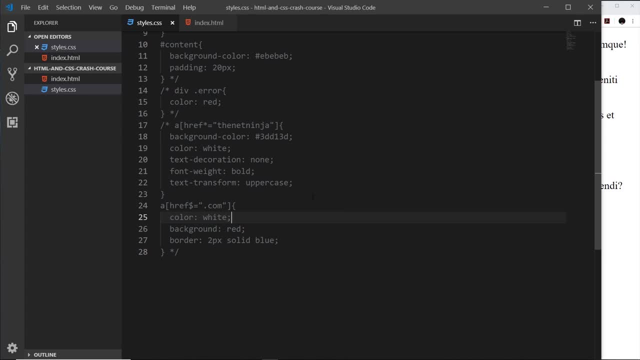 take a look at this text. So I'm going to take a look at this text and I'm going to take a look at this whole inheritance in action. So what I've done is commented out all of the rest of the CSS. So we've 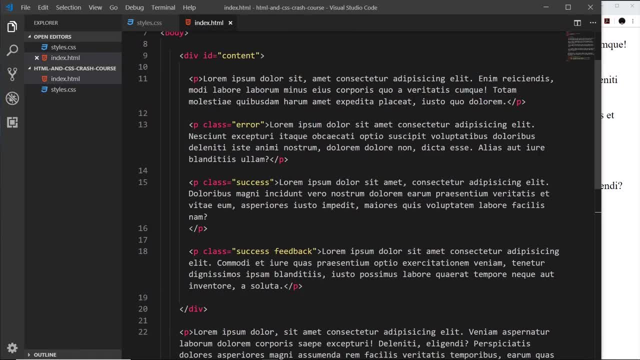 got pretty much a blank slate. The HTML is still the same over here, but it looks like this in a browser because we have no styles applied to it at the minute. So then, my friends, let us now try out this inheritance business. So I'm going to say div to target the divs on the page. Now, look, we have this. 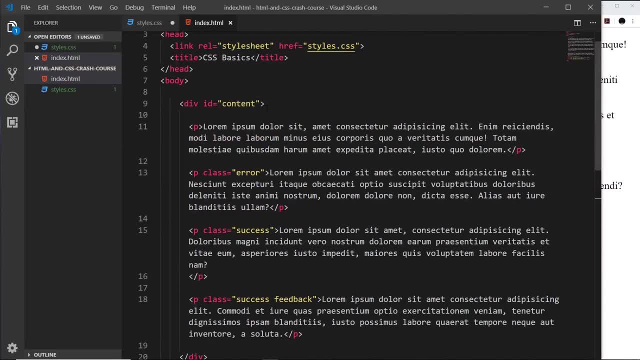 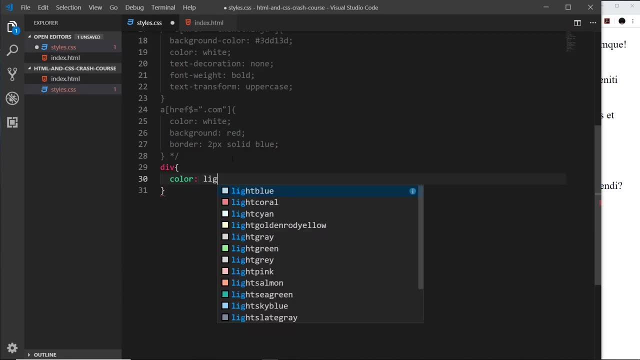 div right here and this div right here. So this one is a parent of all these parents. So I'm going to save that. Now, if I was to say color, and then I'm going to say light coral, It's always nice to have. 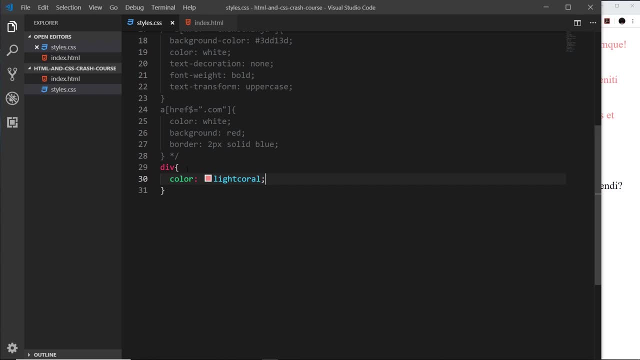 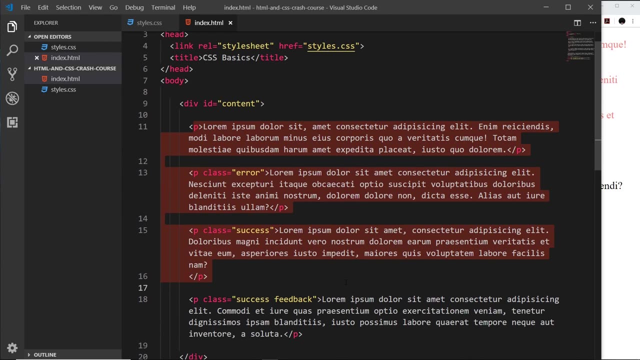 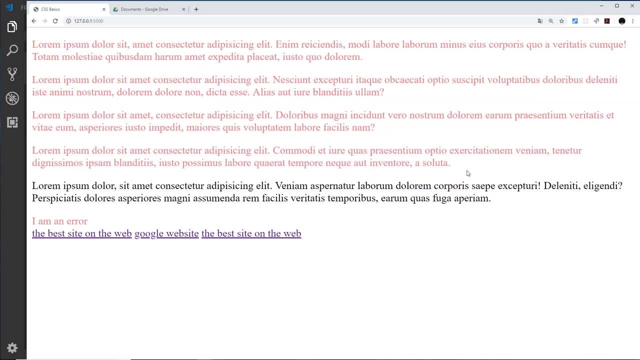 an unusual color. Save that Now, because this is the parents and we have inheritance going on. all of the children right here they are going to inherit this property And you can already see over here on the right we have all of these P's or paragraph tags. They are all colored this coral color. So 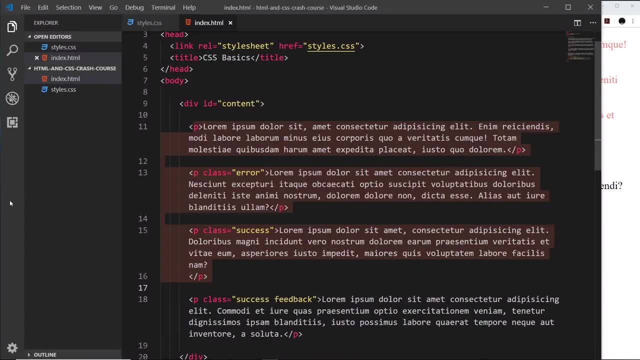 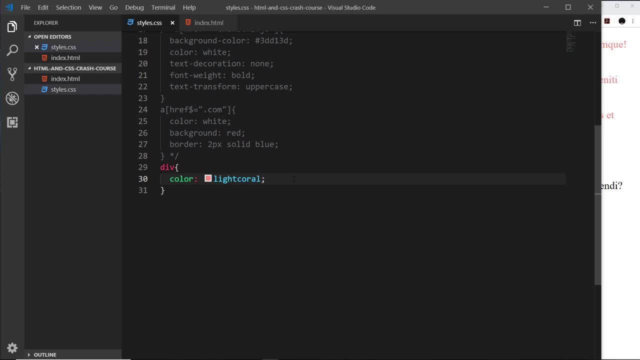 it's inheriting that property. now, Not all properties are inherited. It's mainly things to do with text, you know, like font weight, or you know font family, font size. But if I now come in here and say border and set this to one pixel and solid, 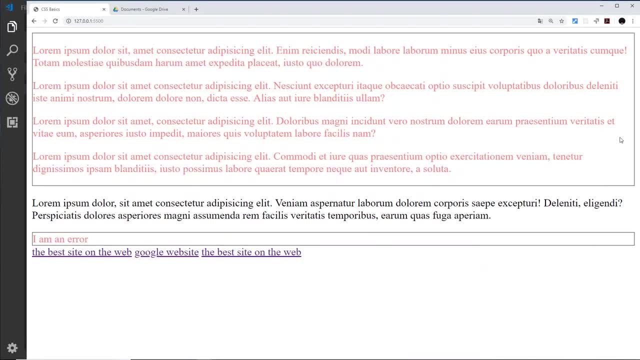 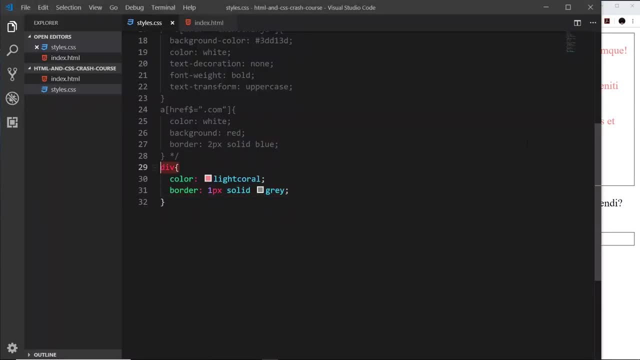 and we'll say: you know, gray, I'm going to save that. Now, notice, that is not inherited. Yeah, the div has this border because we're styling that explicitly right here. the div, But the P tags inside it. they are not getting a border each. No, it's just. 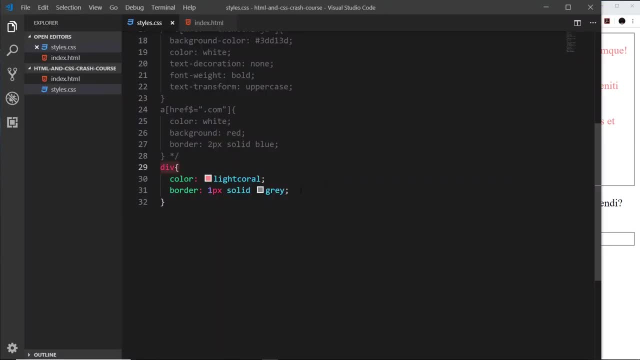 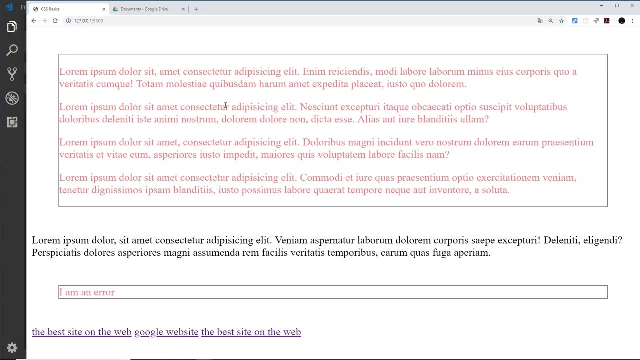 The one single parent div that has the border. Now then if we also do another property, which is margin, and set that to be something pretty big so we can notice it- 40 pixels- Then again the div gets the margin around it, But these paragraph tags they do not. they do not inherit the margin. However, if we 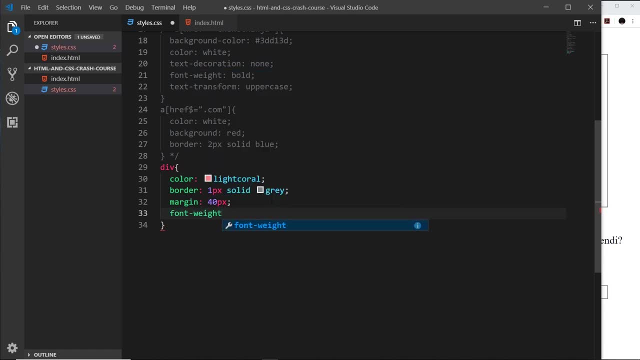 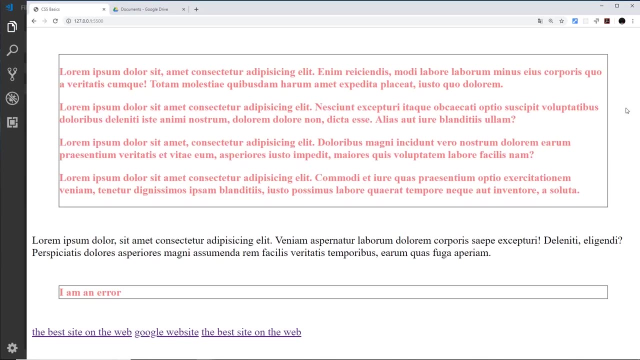 now do something like font, hyphen weight and then set this to be bold. Let me try this out. Save it Now. this is inherited, So again Another style to do with the text. really, that is being inherited by these children, So that 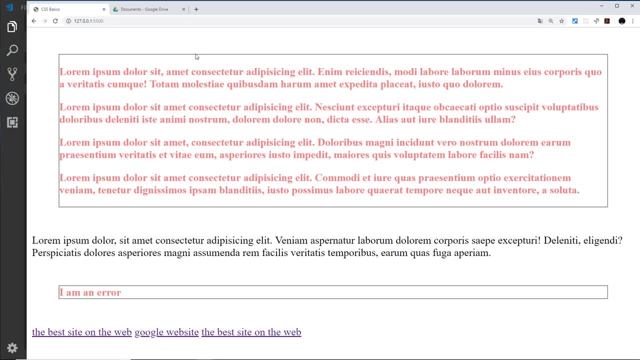 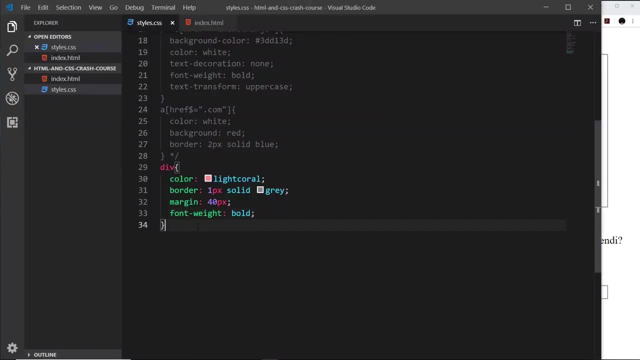 Imagine we want to, as a child of a parent, inherit something that isn't automatically inherited. Well, how would we do that? Pretty simply, actually, we could come down here and say: OK, we have this P tag, and now I want to inherit the values for the border and the margin. I might not necessarily know what. 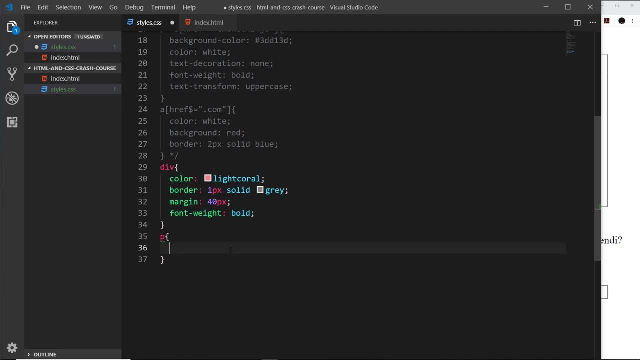 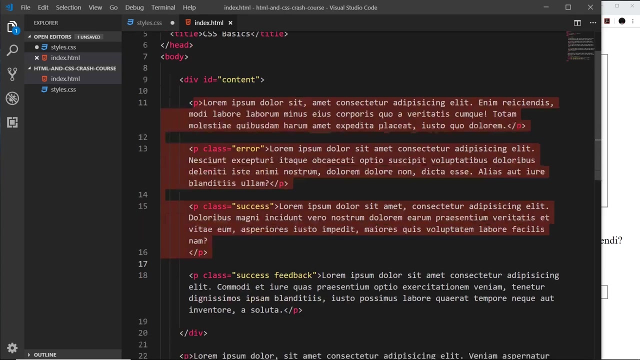 they are. Don't want to write them out explicitly again And I can just say: border Inherit, like so, and margin inherit, OK. So what this is going to do, my friends, is look at the parents of whatever P tag we're currently styling. Now, in these cases, this is the parent, And if we have a style for 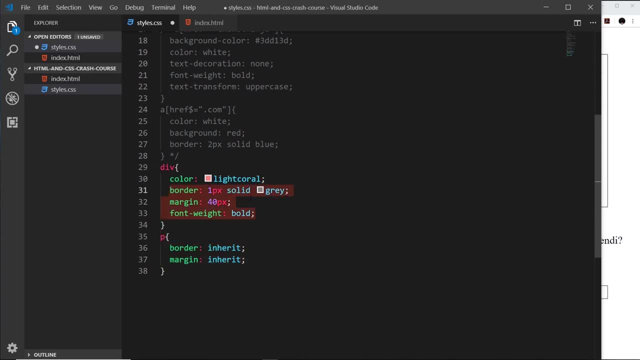 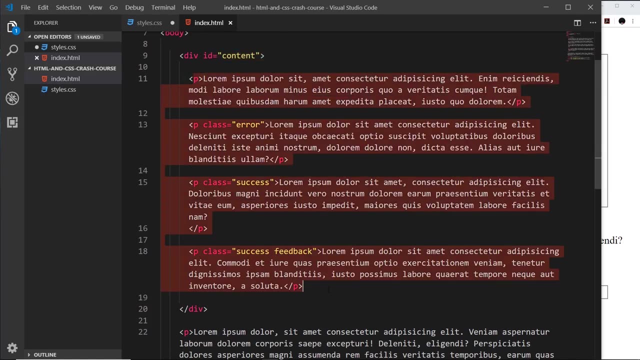 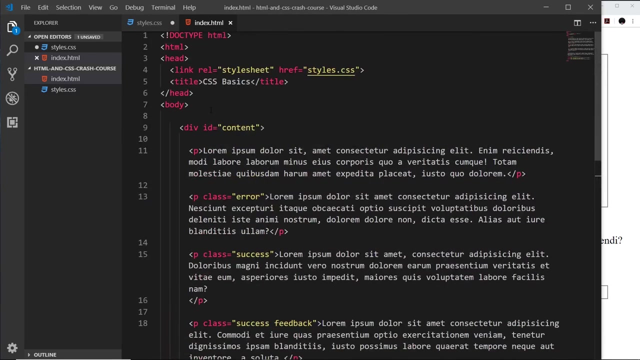 the border and the margin added to the parent, then it's going to inherit the values from those because we said inherit them right here. So that's going to apply in the case of these P tags right here, because this is styled with the margin and border. But this P tag- the parent of this- is the body tag. I. 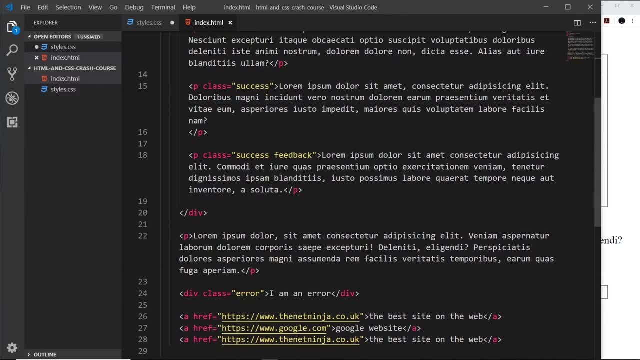 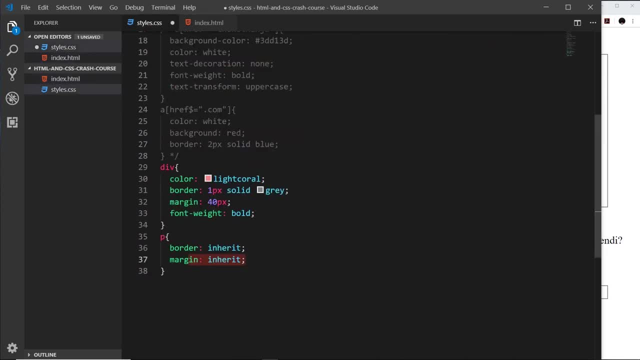 suppose. So that is not going to inherit any of those styles, because the body is not styled with the margin or the border, So only these things are going to inherit it. So if we save that now and preview, we can see now we have a border around each paragraph tag and also that margin. 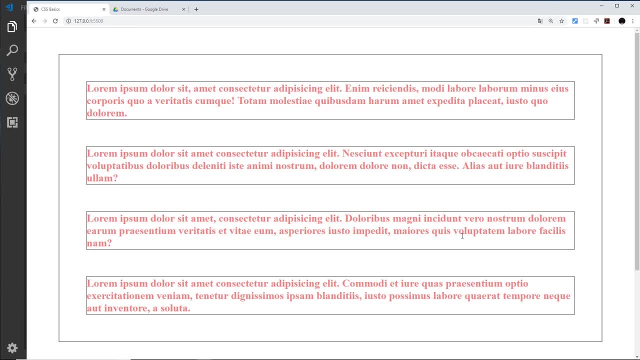 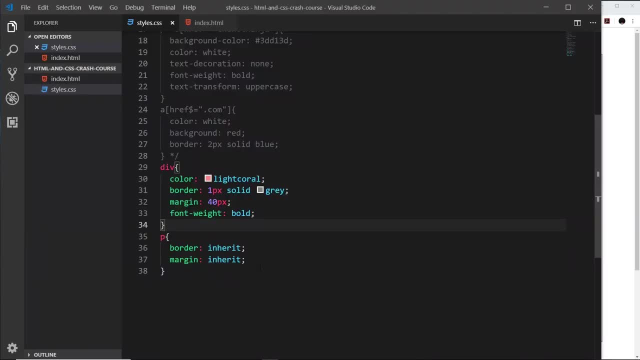 So that's nice. We can inherit things if we want to, even though they're not directly inherited for us. OK, So we have this idea of inheritance and you know, the P tag can inherit whatever is specified right here, And in the case of the color and the font weight it's doing that automatically. Now what if I? 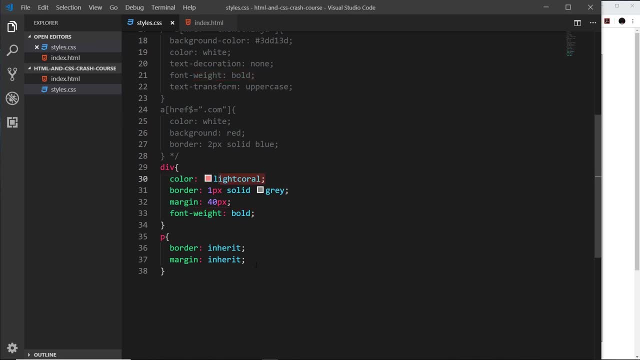 wanted to override the color. So maybe I don't want these P tags to be like coral, I want it to be something else. Well, I can simply just say color and set that to crimson and save it. And now we're going to see crimson text, And that's because this is the color of the text, So you can see that it's. 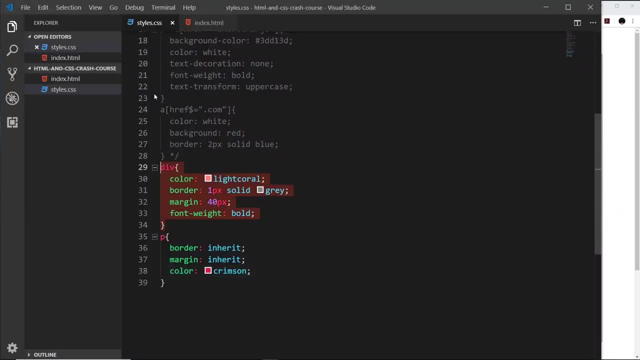 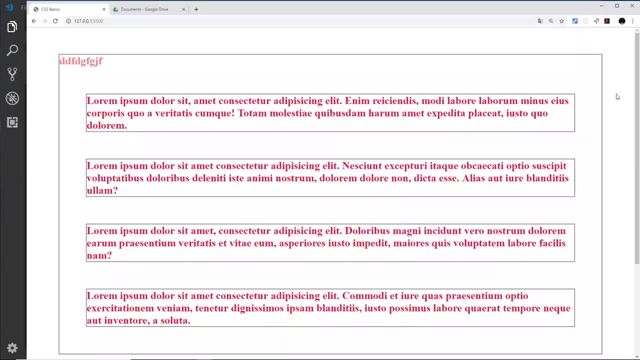 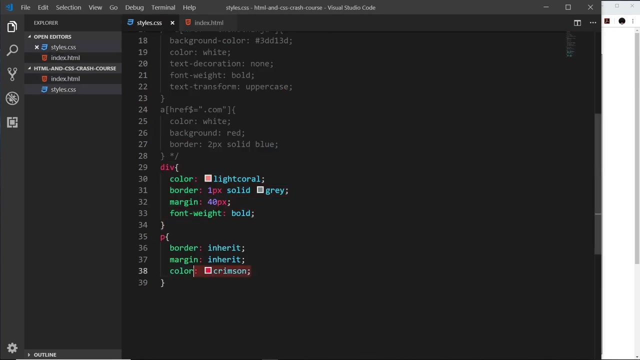 a more specific selector, We're styling the parent, And if we had any kind of text directly in the parents, not in a P tag, then that would still be like coral, as we can see right there. But because now we have a more specific selector for these paragraph styles, it's overriding the 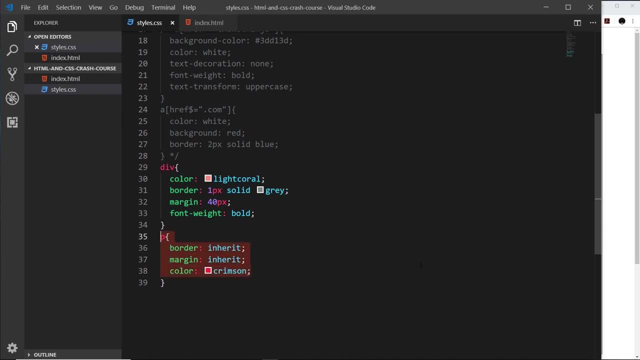 color value. This one is essentially more specific than this one. You know, we're just styling the parent here, We're actually styling the element itself right here. So this brings into the equation the idea of specificity as well, And we can override inheritance. So then now what if I 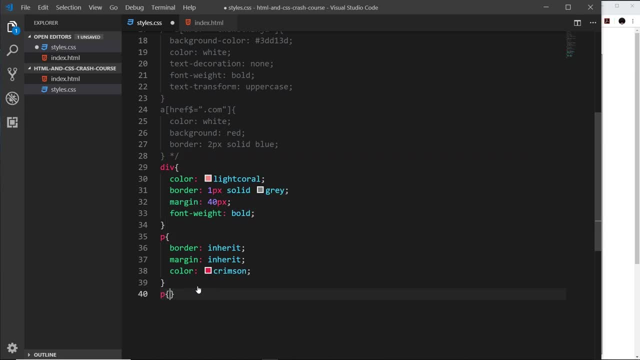 later on, down the CSS file somewhere else, I add another style for the paragraph tag, So I use the same selector. Probably shouldn't do this, But this time I say color is orange. Well, what's going to take precedence then? Well, it works from top to bottom. So whatever is declared last or further, 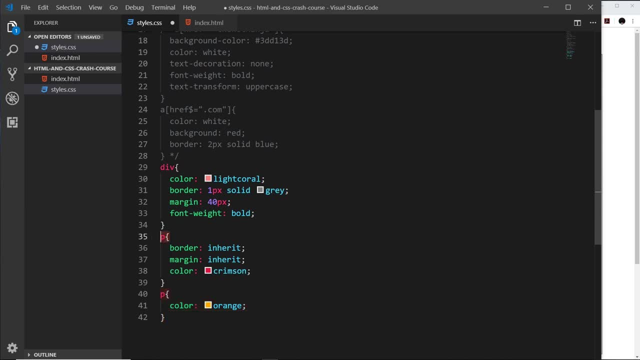 down in the style sheet that takes precedence. So even though these two are the same selectors, when there's a conflict like this, the one that is further down takes precedence. So now it should be orange, and we can see that right here. Okay, But if we're talking about specificity, I could 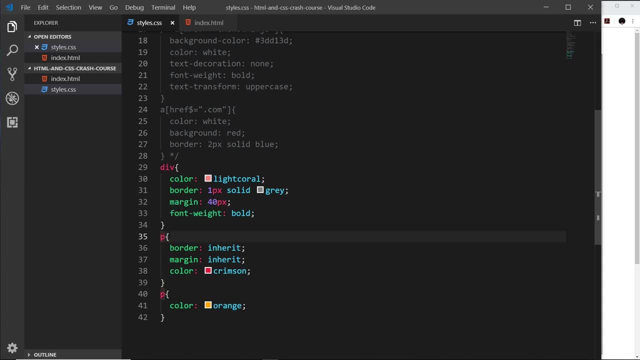 make a more specific selector. For example, I could say div and then space, then P. This is a descendant selector, remember, And this is more specific than this. I know that might seem weird, because we're targeting exactly the same thing, But because we're saying: okay, we'll get all the P's and the 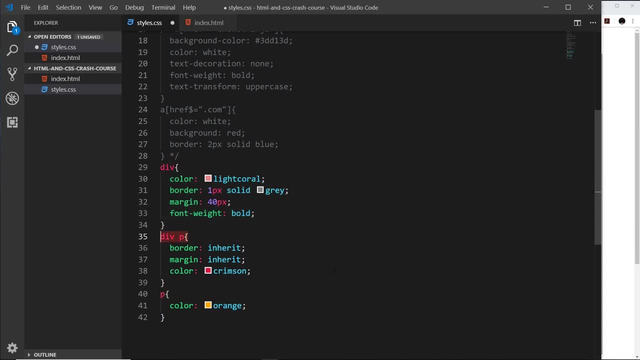 inside a div. This now is a more specific selector. It carries more weight than this And, even though this comes further down in the style sheet, this is now still going to take precedence because the specificity is higher. if you like, It's more weighted. So, if I save it now, we should. 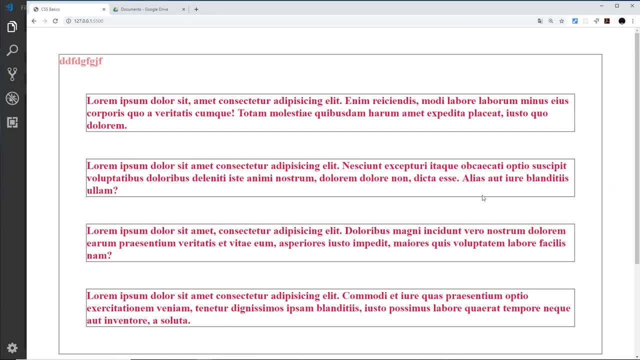 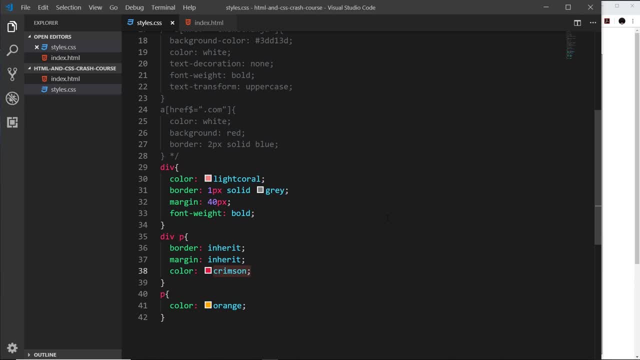 see crimson instead. Okay, so now we can see crimson. So I know this idea of inheritance and specificity is probably going to be quite a lot to get your head around, And you might find yourself playing around with this a little bit And, by the way, I would implore you to do so. 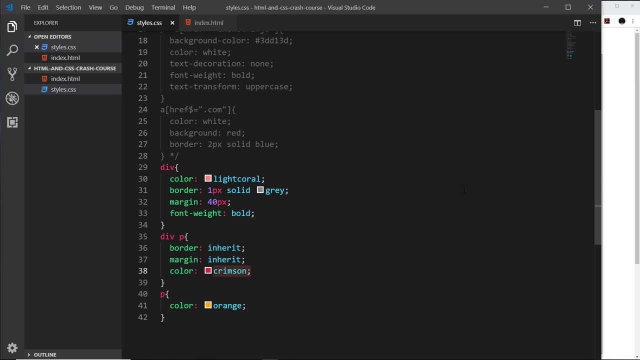 because the only way to learn something properly is to test and test and test things yourself. But also, what I'm going to do is I'm going to leave you a link to a really good article- or guide, rather- on the Mozilla website, all about selector specificity. So I would advise. 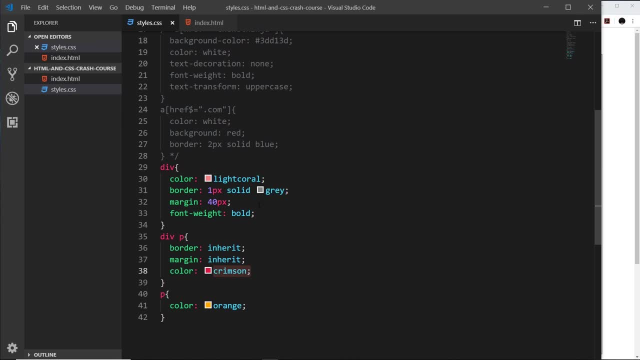 you to read that if you want to understand more about this, because there are many times when you're trying to learn something and you're trying to learn something and you're creating CSS rules and you've got some inheritance going on, And because your style sheets are so big. 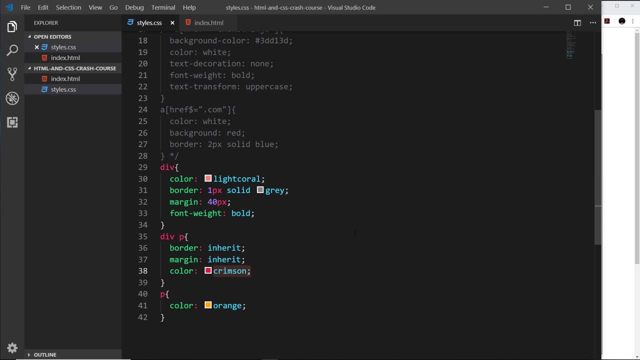 and so many lines long, then it can get a bit messy And you're not sure what elements are inheriting from what and what selectors are more specific than another And it can get a little bit confusing. So definitely check out that article. The link is going to be down below, But hopefully 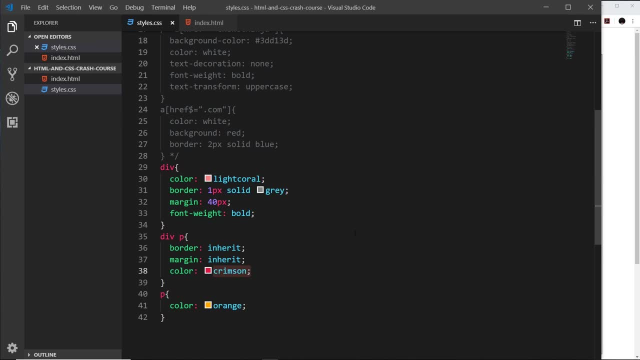 now you have kind of this rough idea of specificity and inheritance, And together they kind of make up this cascade in CSS, And that's what it's all about.